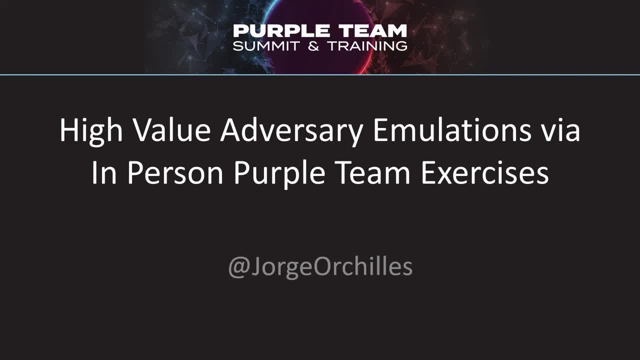 Hello and welcome to my presentation on performing high value adversary emulations via in-person Purple Team exercises. This talk was originally presented at the SANS Purple Team Summit and Training in 2019.. My name is George Orchias and you can follow me on Twitter and. 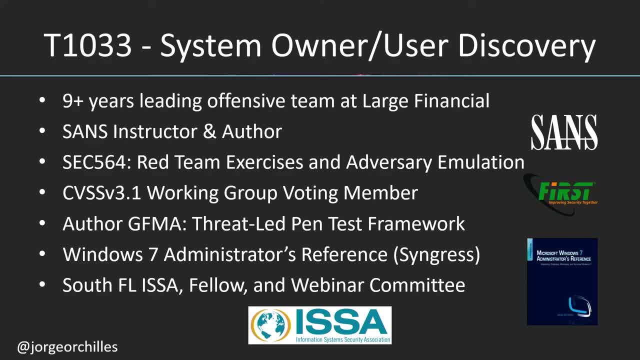 LinkedIn. I've been in offensive security at Large Financial for nine plus years. I am a SANS instructor and author of Security 564, Red Team Exercises and Adversary Emulation. It's a two-day course. If you're interested, check it out at the sansorg site. I'm part of the working group and 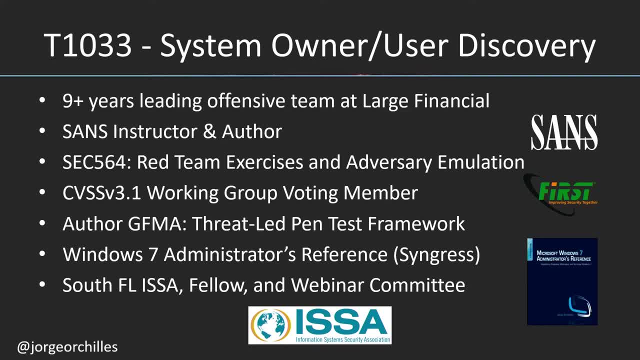 a voting member of the Common Vulnerability Scoring System. I'm also a co-author of the Threat-Led Penetration Testing Framework from the Global Financial Markets Association. I wrote a book in my past life on Windows And I'm heavily involved in the community, particularly the Information Systems Security. 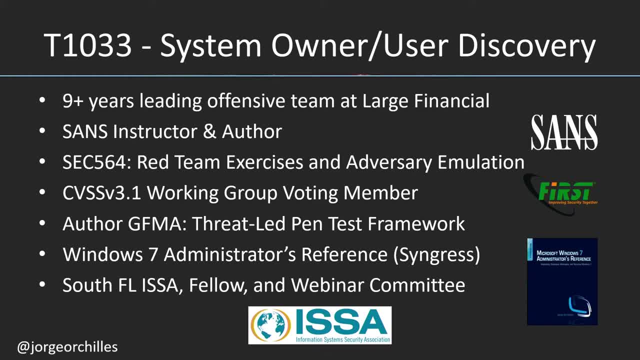 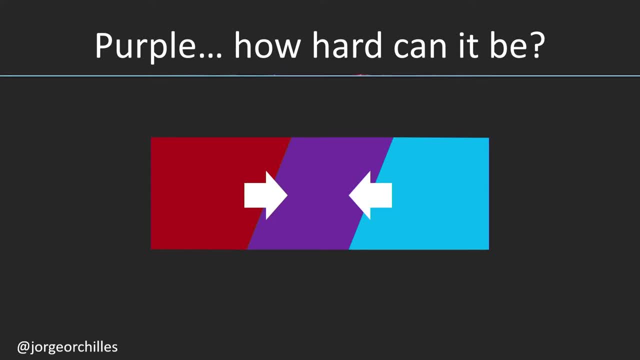 Association. Being a member of the South Florida chapter, I'm also an ISSA fellow and part of the webinar committee. So purple, how hard can it be? I asked my daughter: how do you make purple? She says that's easy, daddy, You combine red and blue. So how hard can it be? You take your red team. 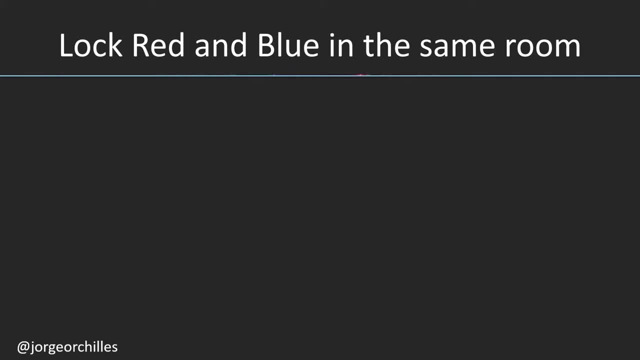 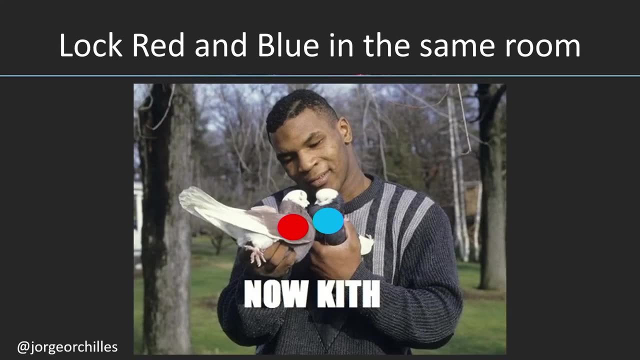 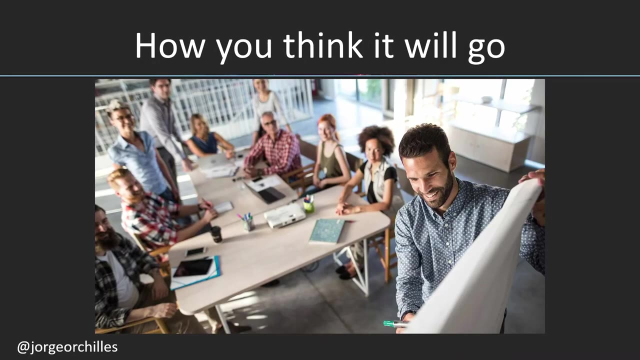 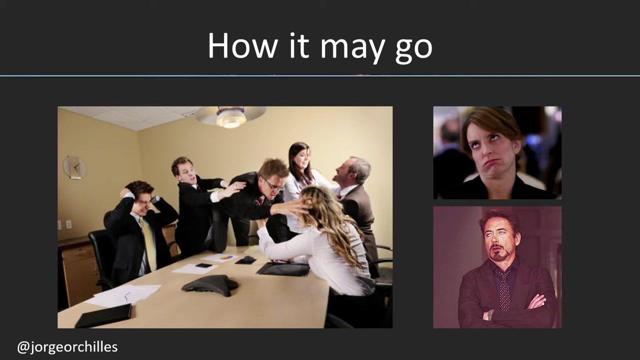 that does offense, and you take your blue team that does defense and you put them in the same room and see what happens. So we think it will go this way, with a lot of people smiling and working together. But it may actually go like this. So what we're going to cover today are the various different 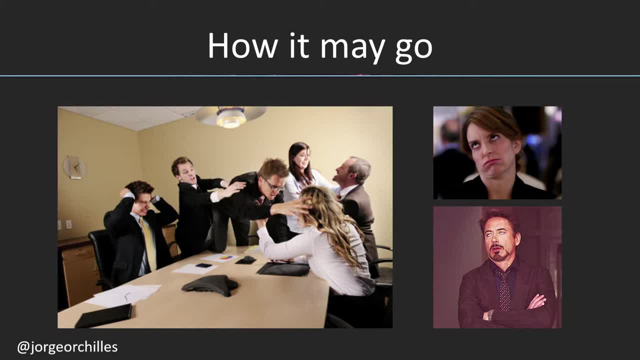 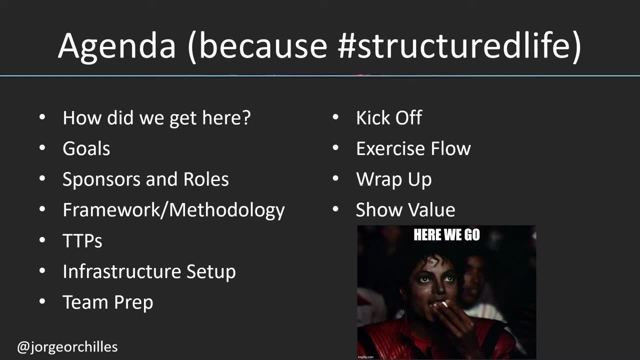 methods and things we've learned in performing in-person purple team exercise. We'll cover why we are doing this And, of course, we'll have an agenda, because structured life. So how did we get here? What are the goals of an in-person adversary emulation? We'll cover sponsors and roles. 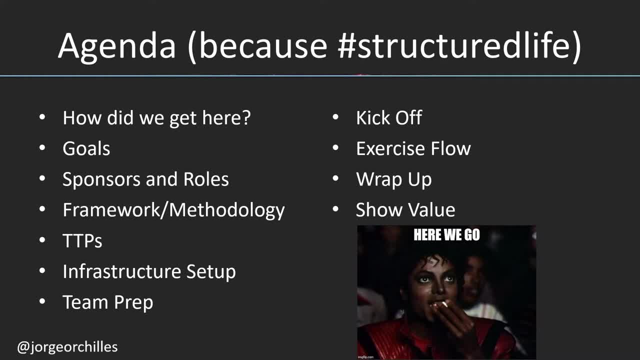 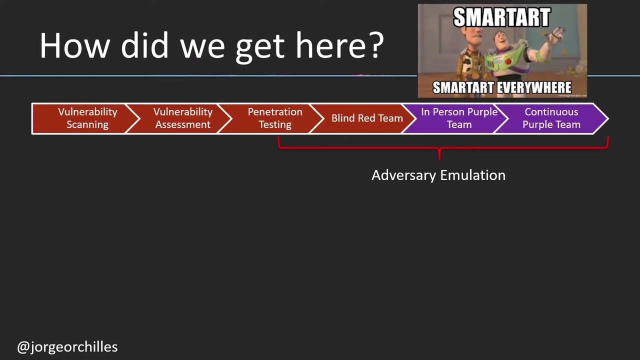 cover frameworks and methodologies. We'll cover tactics, techniques and procedures: Setting up an infrastructure for this, Setting up the various different teams, Kicking off the in-person exercise, Having an exercise flow, Having a wrap-up of the session And then showing value. So how did we get here? We got here. 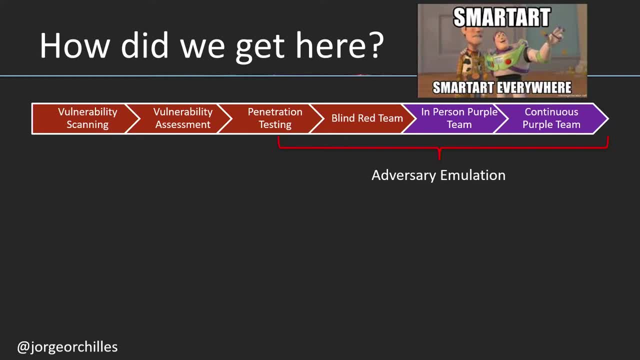 because we started doing vulnerability scanning to identify vulnerabilities. Then we did vulnerability assessment to triage those vulnerabilities and only report issues that really existed, So the system owners would only spend time fixing real issues, not false positives. Then we said we should really. 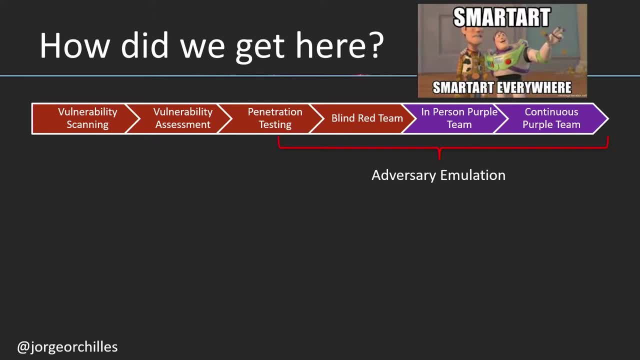 exploit this vulnerability and see how far we can go. Can we determine real business risk And penetration? testing was great for a while until we saw a lot of regulations really scoping and limiting what we can do, And that's where red teaming came along. Red teaming- 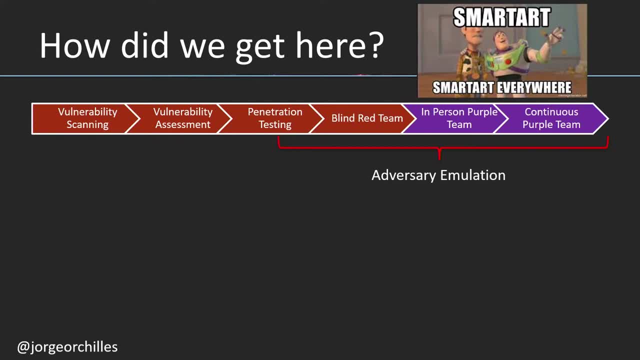 is open scope. very little rules emulating actual adversary tactics, techniques and procedures, most of the time in a blind manner. That means the blue team does not know about it. From there we decided blue teams should know about it, Not all the time, but sometimes. So to get there we did in-person. 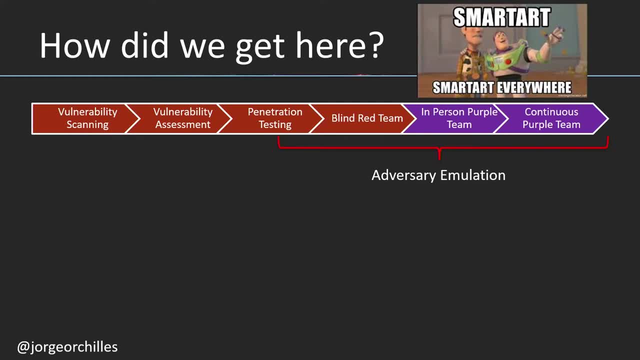 purple teaming. This allowed the red and the blue team to form as a virtual team And then, after we do in-person purple teaming, we did in-person purple teaming And then, after we do in-person purple teaming, we should be able to have continuous purple teaming. So what is adversary emulation? 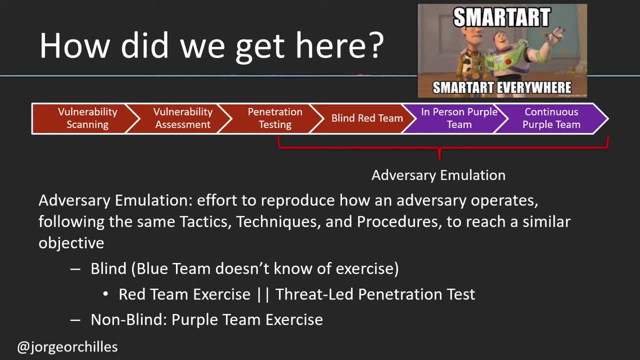 It's an effort to reproduce how an adversary operates, following the same tactics, techniques and procedures, to reach the similar objective. As I mentioned, there is blind testing, often known as red team exercises or threat led penetration tests, And then there's non-blind. 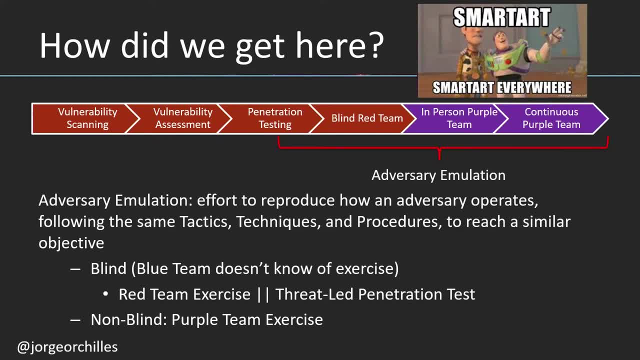 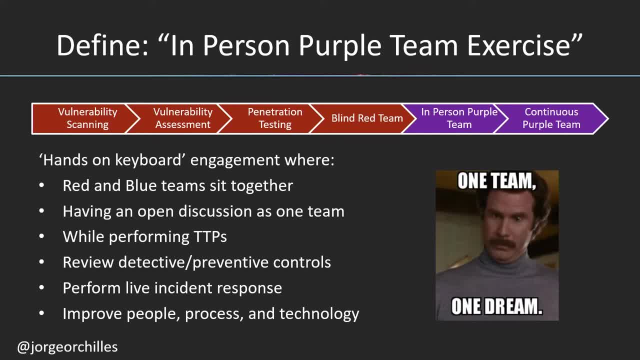 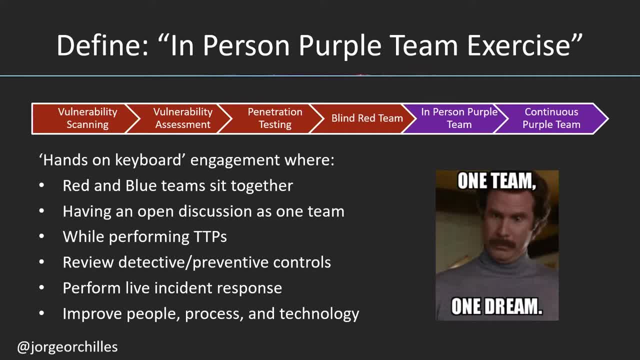 it. So red and the blue team will be sitting together, the offensive team and the security and defense teams. We'll have open discussions. as one team, We will perform the tactics, techniques and procedures that the malicious actors and the red team will do. So we will perform. 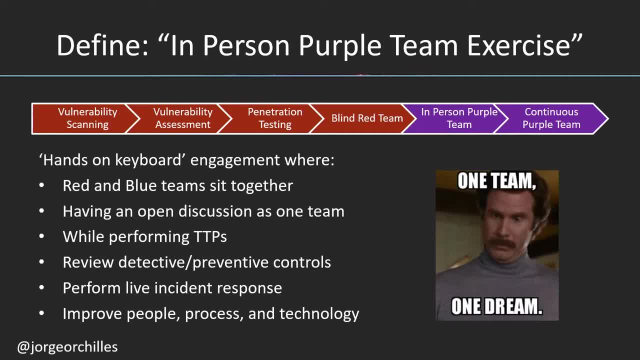 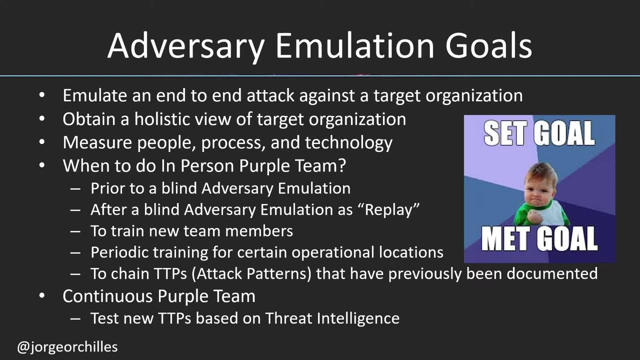 the tactics, techniques and procedures that the malicious actors and the red team will do. So we will review the detective and preventive controls. We'll perform live incident response and forensics and hopefully we improve people, process and technology. So what are the goals of an adversary? 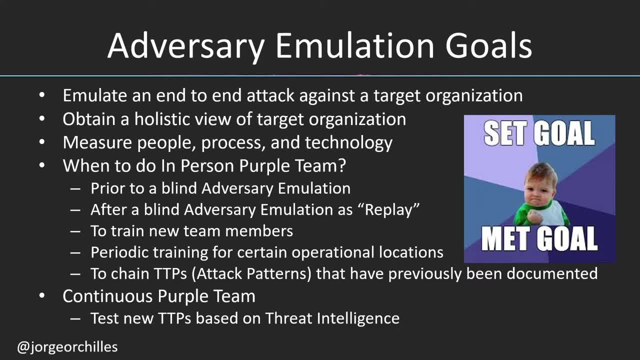 emulation To emulate an end-to-end attack against a target organization. We want to obtain a holistic view of the target organization. We want to measure people, process and technology. When should we do these in-person purple team exercises? Best case scenario, I believe, is to 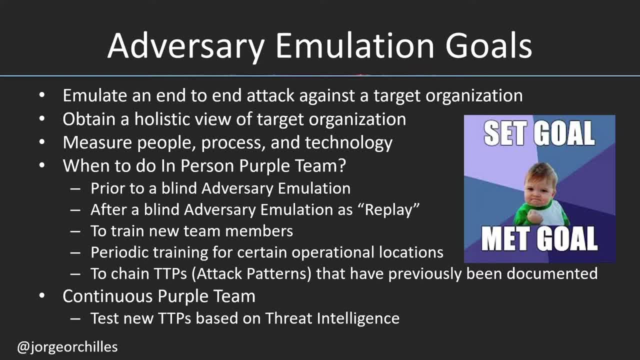 swap them. Do a blind red team engagement, then do a purple team engagement. You cannot do one of these prior to a blind red team engagement, after a blind red team engagement, as a replay If you have new team members in your security operations center or in your incident response team or in. 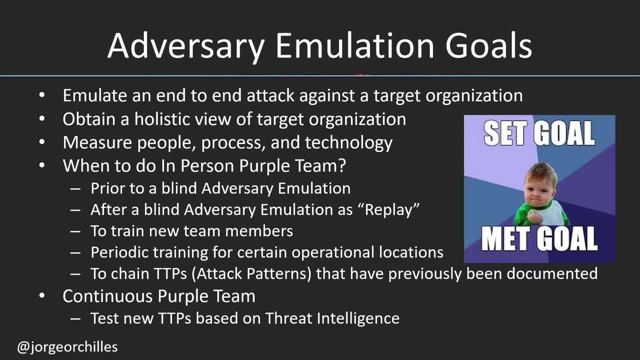 your forensics team. it might be a good idea If you want to do periodic training for the certain locations or if you want to chain various TTPs that haven't been previously documented. And then, of course, you want to get to a continuous purple team state Whenever a new tactic. 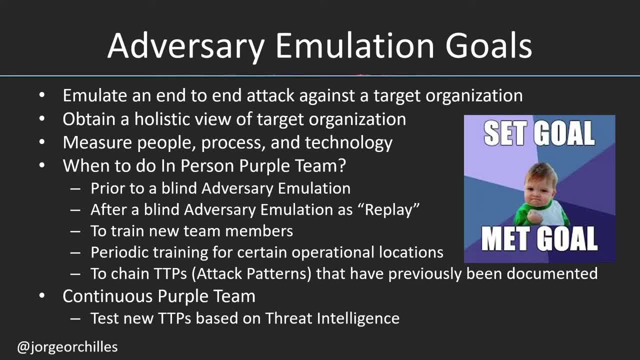 technique or procedure is released, say at Black Hat or DEF CON or HackFest, you want to be able to work quickly together to build a detective and prevention around that particular TTP. So let's talk about doing an in-person purple team exercise. Well, first of all, we need sponsors, because we're going to need 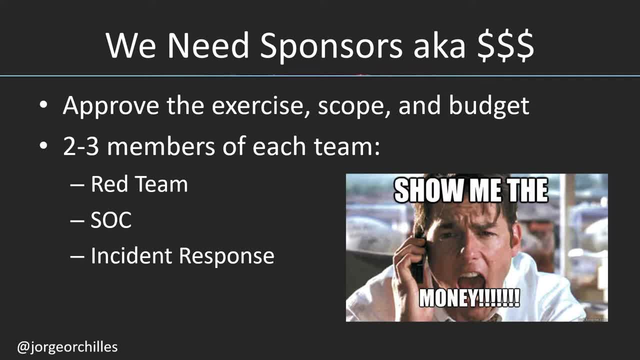 team members from the red team, from the blue team, incident response team, hunt team and generally we have two to three members of each team. That means we have to take them out of their day-to-day job for one to five days, move them all to a location, which means we need a budget. 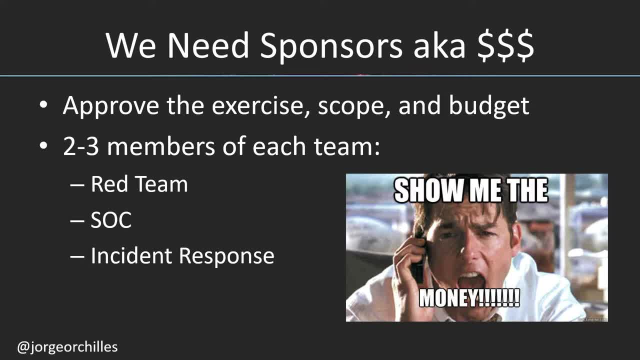 and then we want to use a good, good scope. We want to do TTPs that really matter. So we need sponsors, Generally someone senior, depending on your organizational structure- maybe the chief information security officer, the head of information security or cybersecurity, really depends, But someone has to sponsor this. 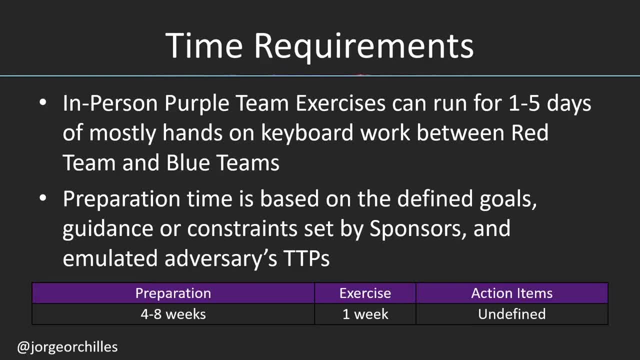 and someone that can approve a budget For time requirements generally. I've seen an in-person purple team exercise run one to five days and it's mostly all hands-on keyboard work between red and blue teams. Now that's the in-person part. The preparation can take a number. 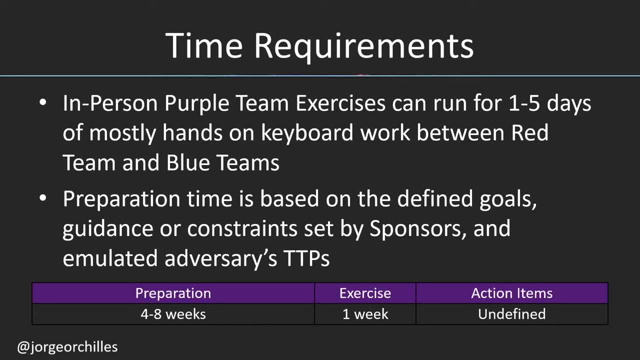 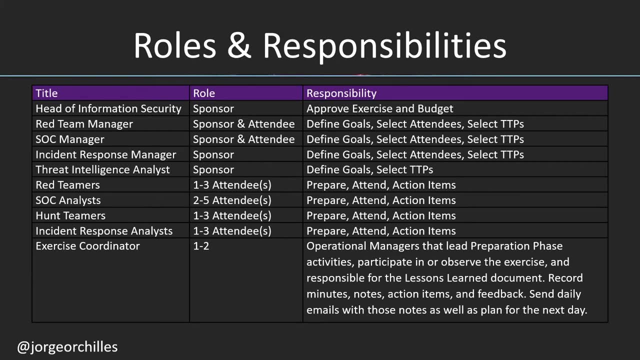 of weeks before that The exercise, just one week- and then the action items of what needs to get done. what needs to be fixed really depends on what you've learned in this particular exercise. Here I've defined the roles and responsibilities for a large organization: the head of information. 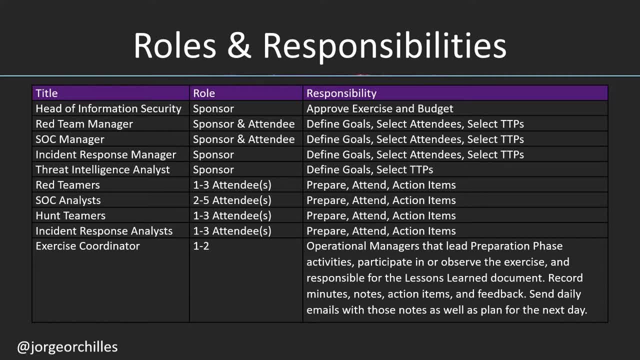 security or the chief information security officer and then the head of information security. The red team manager is a sponsor and generally an attendee. They should define the goals, select the attendees and select the tactics, techniques and procedures. Same for the SOC. 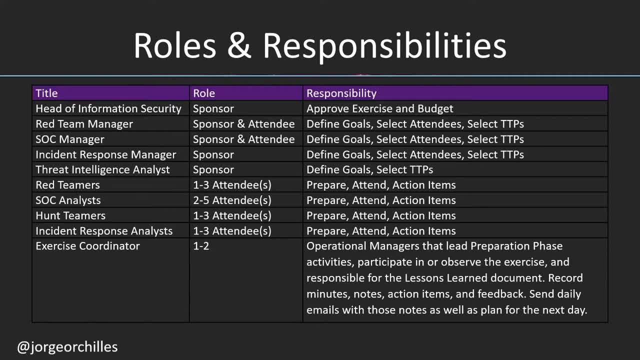 manager, The incident response manager and the threat intelligence analyst should also play a part. Most of the time they are not part of the exercise as they don't have hands-on keyboard, but it really depends on your organization. Then you have a number of attendees, from red teamers to SOC analysts to hunt teamers. 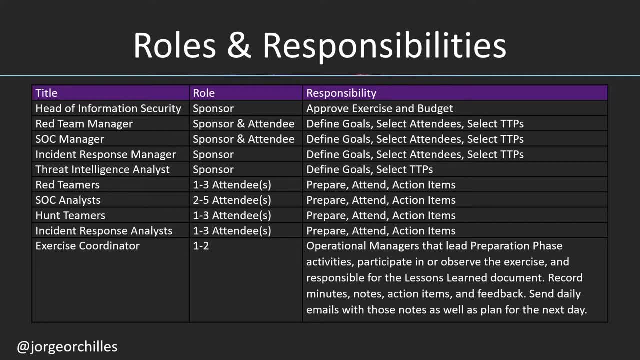 to incident response. And then, lastly, you need an exercise coordinator. I cannot stress this enough. You should have one or two people that are not any of these other roles, that are actively participating and observing, taking notes, writing lessons learned, recording minutes. 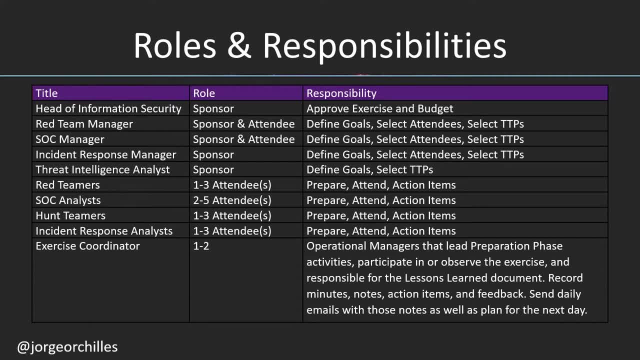 taking the action, And then you have a number of attendees, from red teamers to SOC analysts, taking the action items and taking the feedback. They'll also be responsible for sending a daily email with the status of what occurred to all the sponsors that are not in attendance but want to. 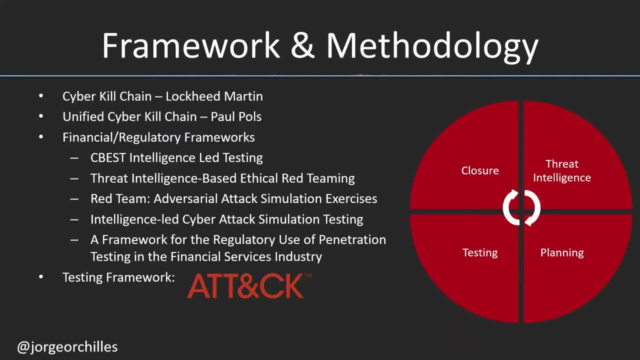 know that their money is being well used For frameworks and methodologies. if we're emulating a malicious actor, we should use a framework that is known. The cyber kill chain is probably the most known one by senior management. I am a fan of the unified cyber kill chain by 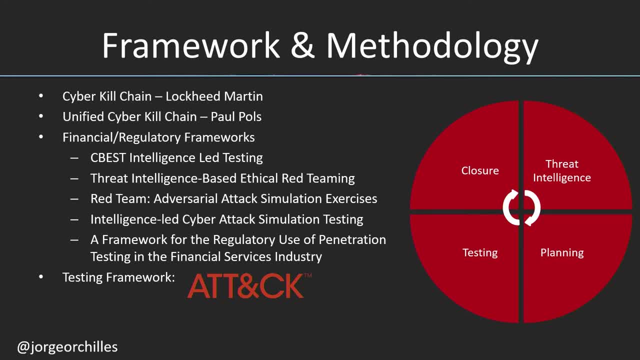 Paul Poles. And then there are some financial and regulatory frameworks as well, from Bank of England to Hong Kong, to Singapore, etc. And then the Global Financial Markets Association released a framework for the regulatory use of penetration testing in the financial services industry. that 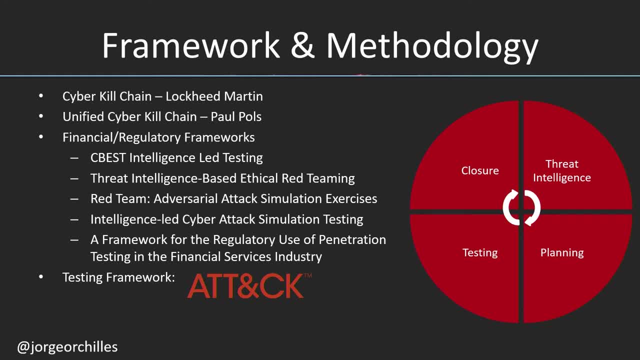 covers all of these regulatory requirements. It's a great framework, so you have a plan of what you're going to do during this adversary emulation. It's not just about running a red team, engagement or testing and hacking. You have threat intelligence, You have to plan, You have to test And then you have to close the exercise with response and 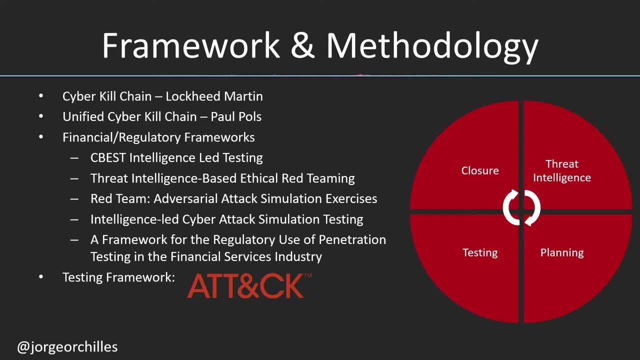 analysis. We're going to cover all of these in this talk. Lastly, for the testing framework, we will use MITRE's ATT&CK Adversary Tactic Techniques and Common Knowledge. So here's our mandatory MITRE ATT&CK slide. We have on top our 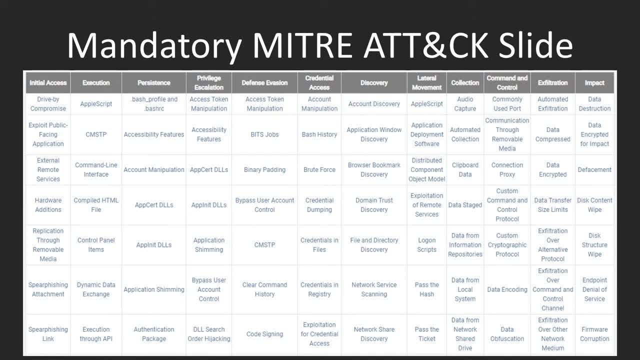 framework for the regulatory use of penetration testing, And then we have a framework for first row are the adversary tactics. These are their goals: Initial access- getting in executing some sort of code, persistence or maintaining access privilege. escalation from a standard user to an administrative or root level user, evading defenses, accessing credentials. 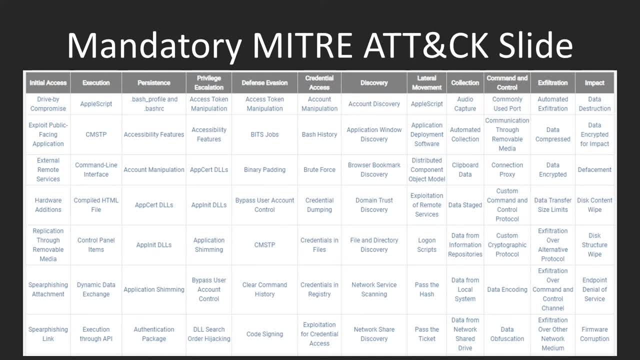 discovery. Once you land on a new system, you should discover things about that host, about the network, lateral movement, And then collection, exfiltration and impact. All of those are action on objectives. You also have command and control, which really facilitates all of these. So those are the 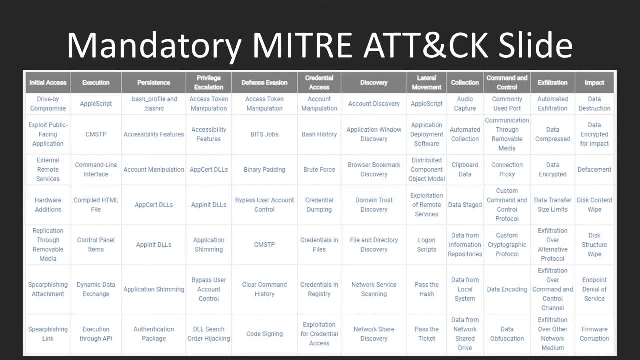 tactics. The top row are the tactics. Everything under it are the techniques. These are various different techniques. There's over 200 of them that have been observed by adversaries using them. You can click on any of these techniques and find certain procedures. There is 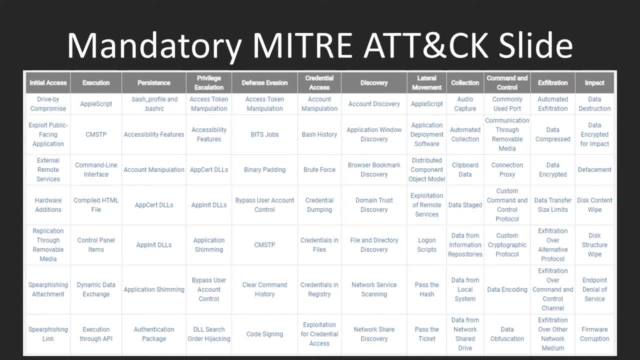 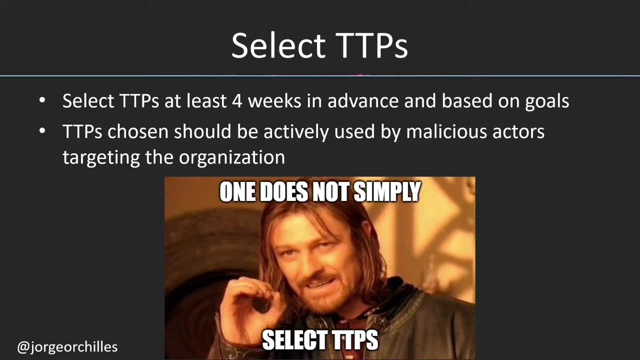 not going to be a hundred percent coverage here. There are many ways to do a single technique, So our next step is to select the tactics, techniques and procedures. This is one of the first things you want to do: to plan an in-person exercise, because this will determine everything. 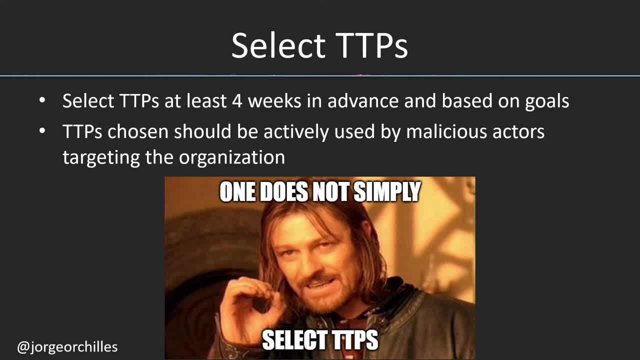 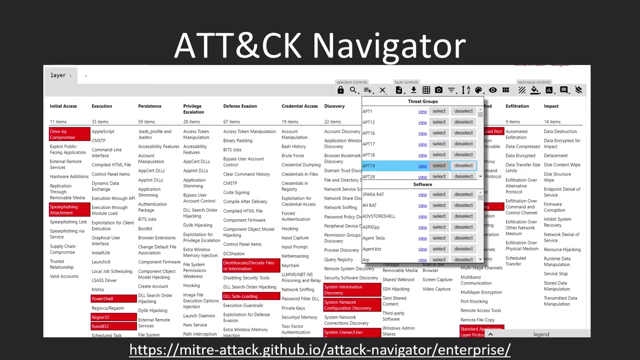 else we're going to discuss in this presentation. They should be tactics, techniques and procedures that are used by malicious actors that are likely to target the organization, An adversary that has the capabilities, the opportunity to do it. So how do we select TTPs? Well, one of the methods is to use MITRE. 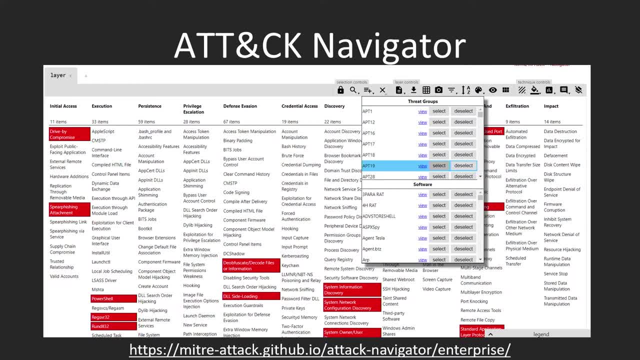 Attacks Navigator. Here on this screenshot, you can see I'm using the selection tool in the middle of the screen and selecting a threat group. In this case, I chose APT-19.. If it, APT-19, is likely to target your organization, These are the tactics and techniques that they 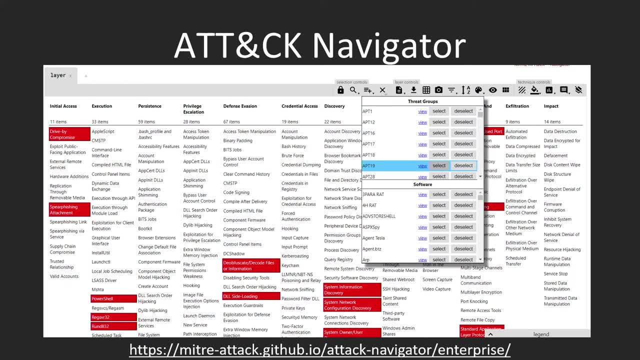 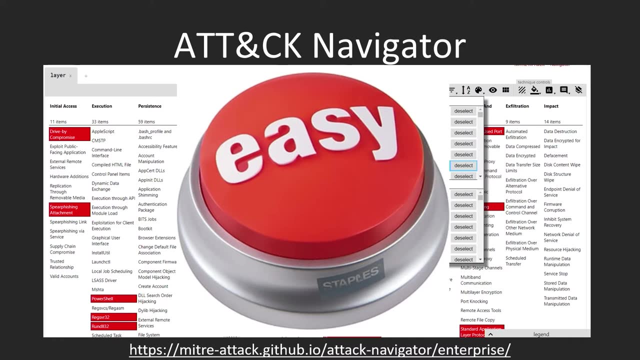 will most likely employ against you. So if that's who you're going to emulate, this is a great way to select this very quickly and have a list of TTPs that you might want to try against yourself, But that's extremely easy. How do the cyber threat intelligence folks and the red teamers really do? 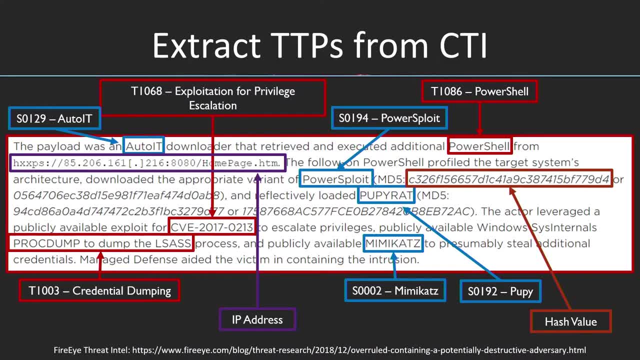 this. Well, they extract TTPs- TTPs from cyber threat intelligence. This screen: you have an example from a FireEye report with the source there on the bottom that says a payload was an auto IT downloader that retrieved and executed additional PowerShell from a website. Just in that one sentence you have a software. 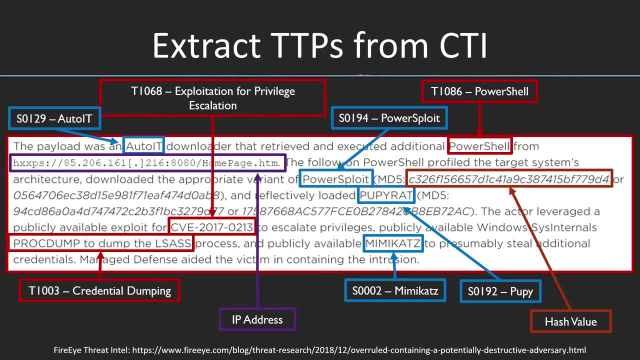 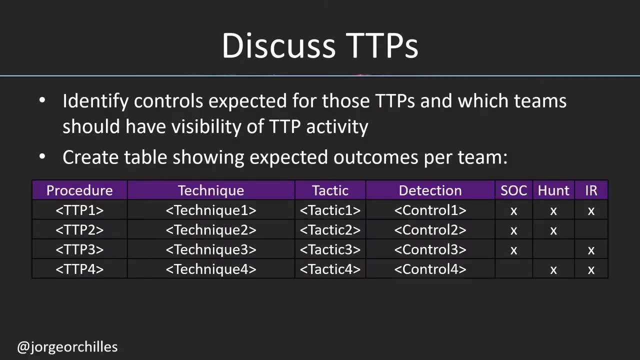 which is part of MITRE Attack as well. software 0129.. You have PowerShell, which is a technique, and you have an indicator of compromise here with the IP address, So you can read all This threat into an extract those TTPs yourself, with a list of TTPs You will then want to discuss. 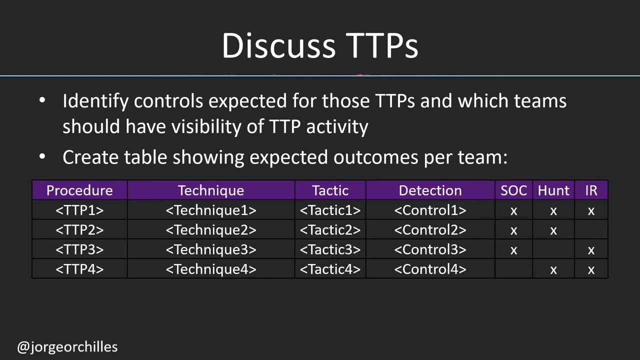 these TTPs between the red team manager, the SOC manager and the cyber threat intelligence person that provided this, to determine which ones they think they have visibility on. Does the SOC have detection for this command and control Channel or do they have detection for PowerShell? Does the hunt team have a test case where they go? 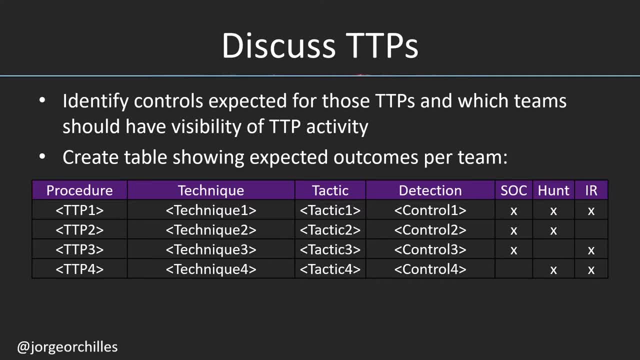 out and they hunt for PowerShell. Does incident response have a method to look at memory and look at our artifacts left behind and determine that particular technique and procedure? The reason you do this is you don't want to go into an in-person purple team exercise with zero visibility. If you 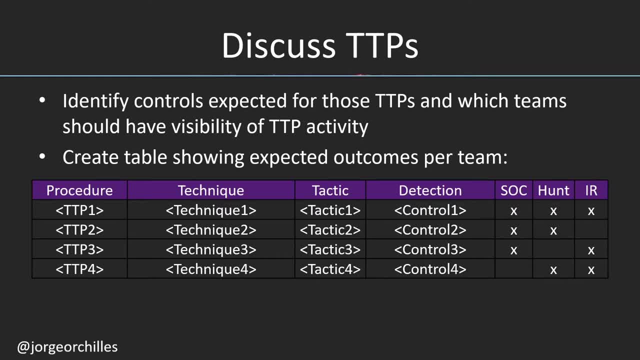 do zero visibility. you don't want to go into an in-person purple team exercise with zero visibility If you do zero visibility. you don't want to go into an in-person purple team exercise with zero visibility. you don't want to go into an in-person purple team exercise with zero visibility If you. 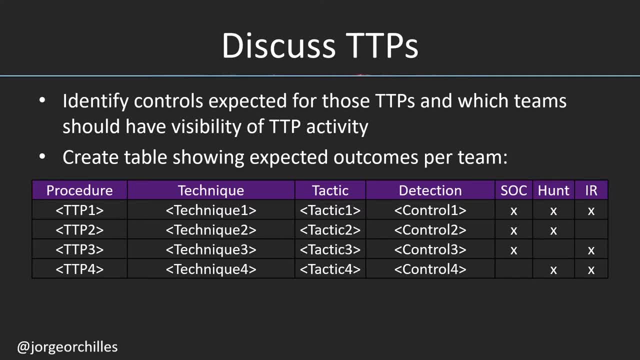 do zero visibility. you don't want to go into an in-person purple team exercise with zero visibility. If you don't look this part of that picture on each one of the drivers, the graphics will be only visible for this one driver. You're not really going to train the people or the process. 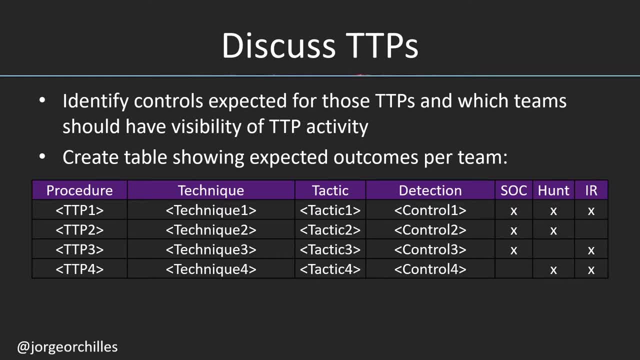 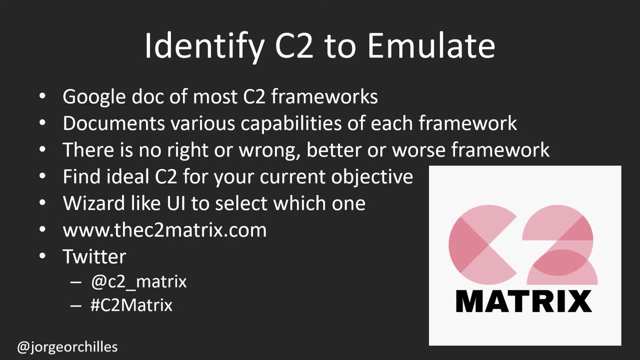 you're probably going to focus on a lot of technology gaps and that's not the point of this particular exercise. You want to identify tactics, techniques and procedures that there is visibility. Maybe some things are prevented, but mostly things are detective and should be alerting. Then you 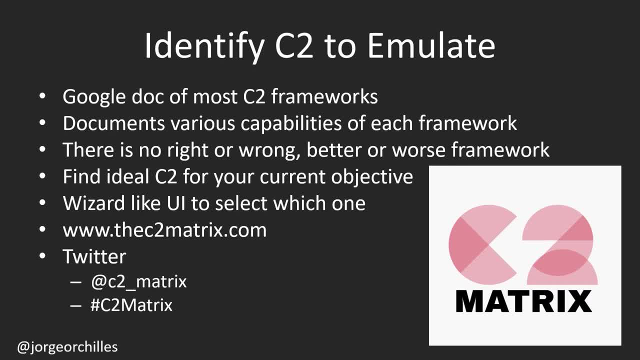 And this is a project I started called the C2 Matrix. It's a Google Doc of most command and control frameworks. It documents their various capabilities and features so that you can choose which framework best emulates your attack. There is no right and wrong. There is no better or worse framework. 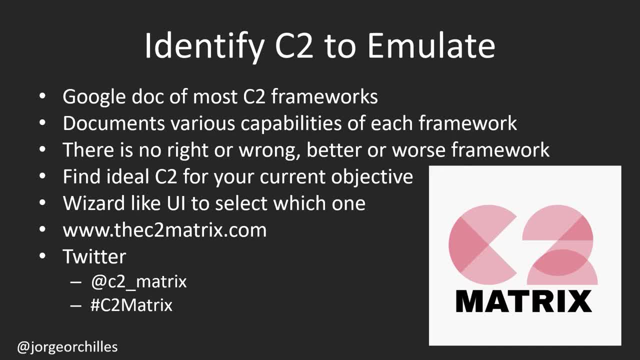 Shout out to all the developers: Thank you for everything you've done. What it does is: it helps you find the ideal command and control for your current objective. It even has a wizard-like UI at askthec2matrixcom. It has a GUI at wwwc2matrixcom. 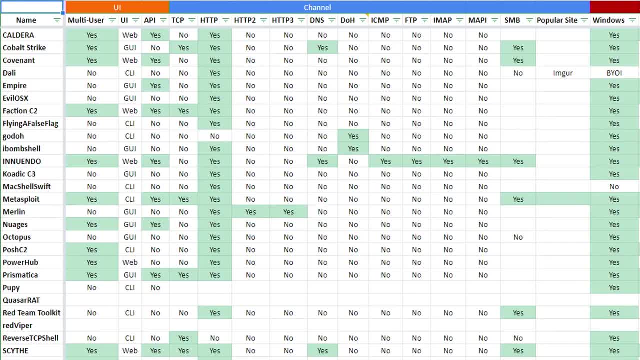 Of course, it's on Twitter at C2 underscore matrix. So what does it look like? It's a Google Sheet with all the C2s on your left and then various different features. The screenshot only shows a few of them, For example, the UI. 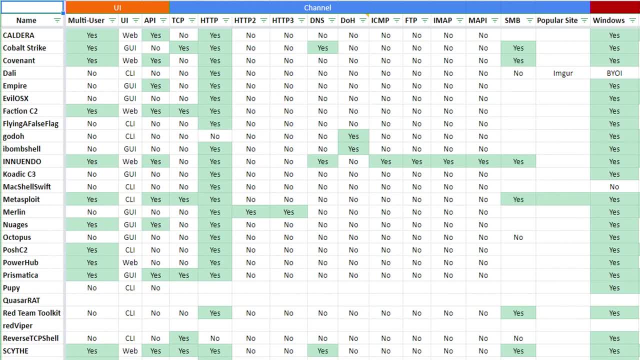 Is it multi-user? Is it only one person can use this framework at a time, or multiple users? How many users can use that instance at a time? How is that UI and does it have an API? Then on this screen you can also see the channels. 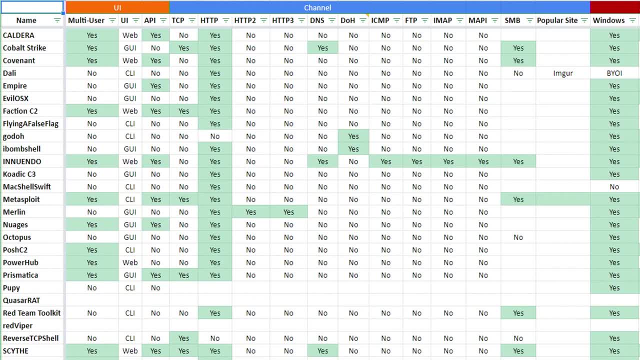 What channels do we allow Or does that framework allow? As you can see, most of these frameworks allow HTTP, But if you want to test some other frameworks, then you can choose which one works best for you. As you scroll through here left and right, there's a number of other features and capabilities that have been documented. 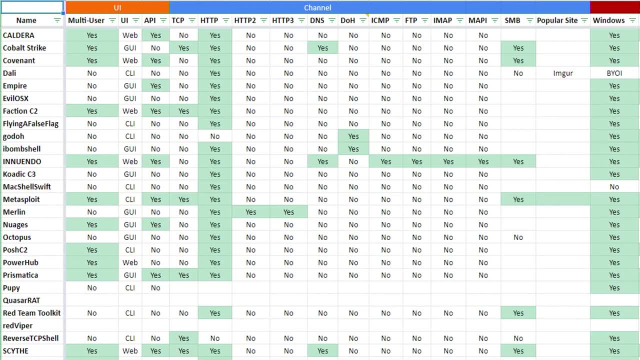 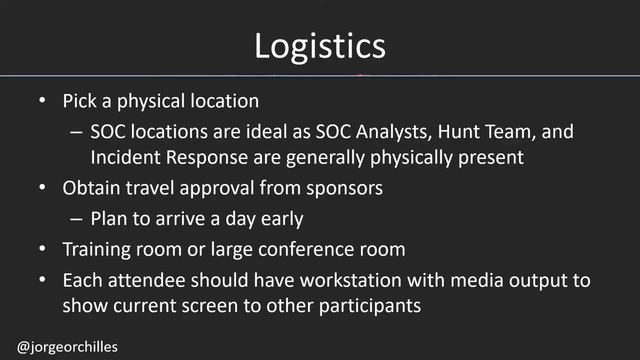 Also shout out to all the contributors for C2 Matrix. Really appreciate everyone that has provided and evaluated and developed some of these C2.. We are open for feedback and contributions. With the C2 selected, you can now go into logistics. As technical people, we rarely think about these things. 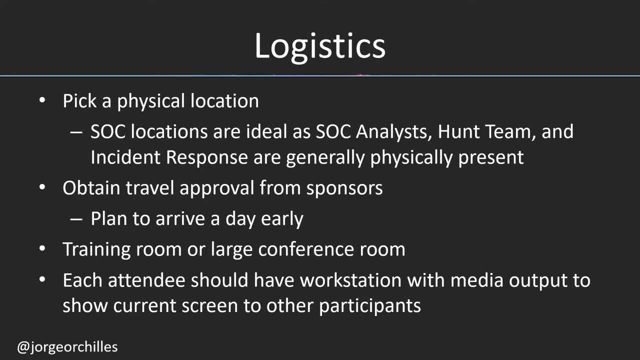 So let me briefly highlight some of the things you need to consider. For example, you need to pick a physical location so that everyone can see. You need to be able to sit in person. Now, that sounds a lot easier said than done. You want a location where you have the least amount of travel. 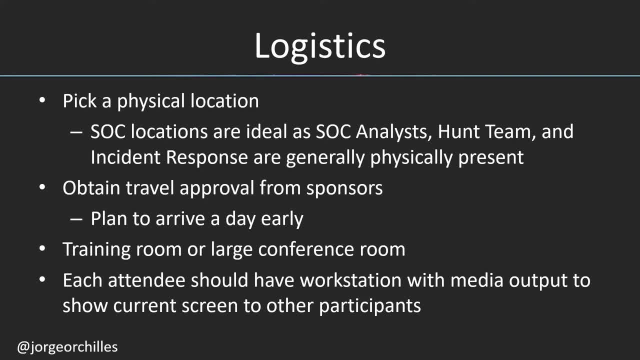 Generally, the security operations center is an ideal place. Maybe you only have people from the hunt team and incident response and the red team flying into there. It really depends. Then you need to obtain travel approval from sponsors. If you're not used to flying with your organization, then this is something you need to do. 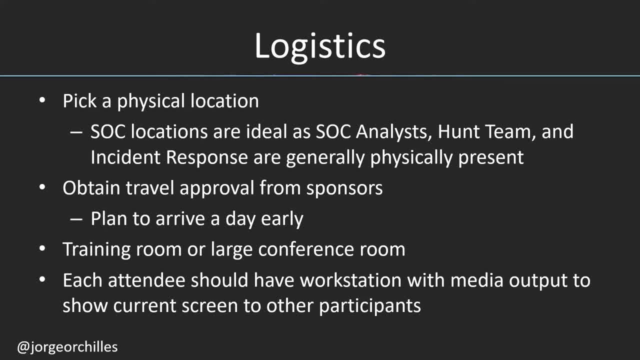 Then you need to obtain travel approval from sponsors. If you're not used to flying with your organization, then this is something you need to do. If you're not used to flying with your organization, then this is something you need to do. Consider: Always: plan to arrive a day early. 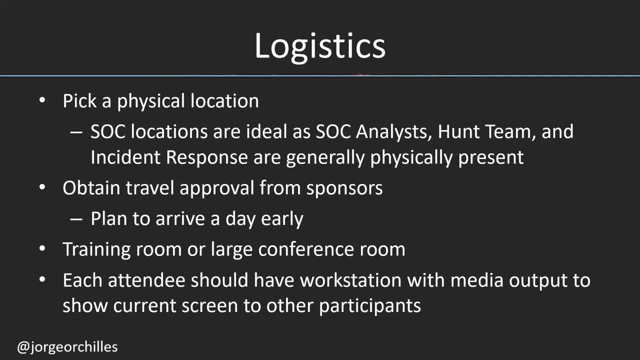 Consider: Always plan to arrive a day early. Then you want to choose a large conference room that has proper connectivity power for all the laptops. Then you want to choose a large conference room that has proper connectivity power for all the laptops, Since everyone will have a laptop. 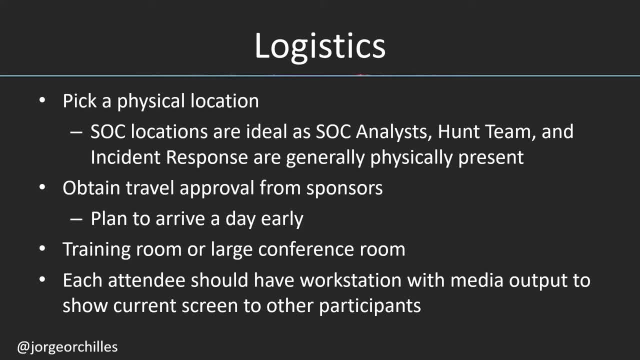 A screen that everyone can share their workstation on, with the same media output, generally HDMI, And that has cooling as well. Generally, these conference rooms aren't used to having that many people. people especially with laptops running and then from there make sure that they can access. 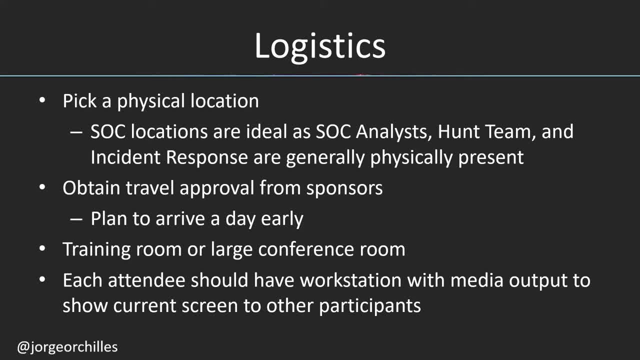 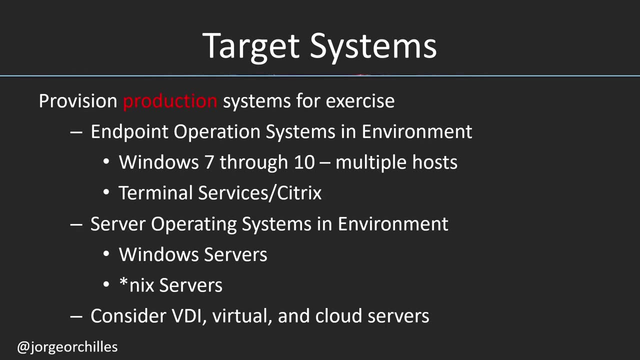 everyone's infrastructure, that the red team can access their target environment, their attack infrastructure, environment that the blue team can access, all everything they need to do their job. then we're going to need some target systems. highly recommend you provision the productions, these systems in production. i'm not saying take over current production systems, but create systems. 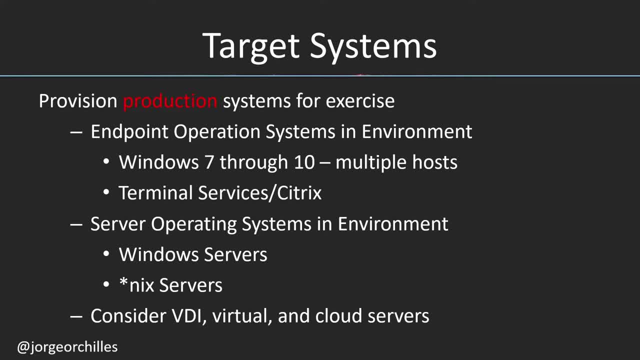 in production, because that's where the visibility is. so if you're targeting endpoint operating systems, get the same operating system with the same configuration, same security tools as your current environment. i'm assuming by now most people are off of windows 7, maybe on windows a or windows 10 if they have terminal services, citrix, vdi, environments, cloud. 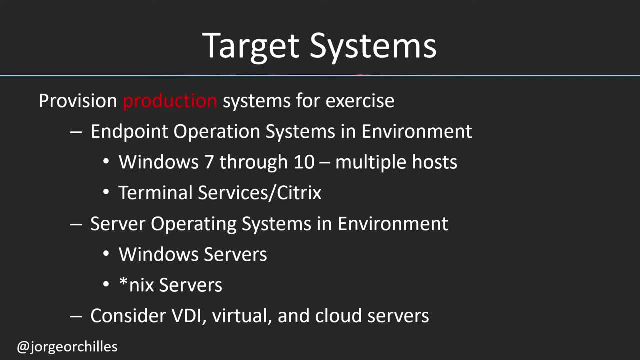 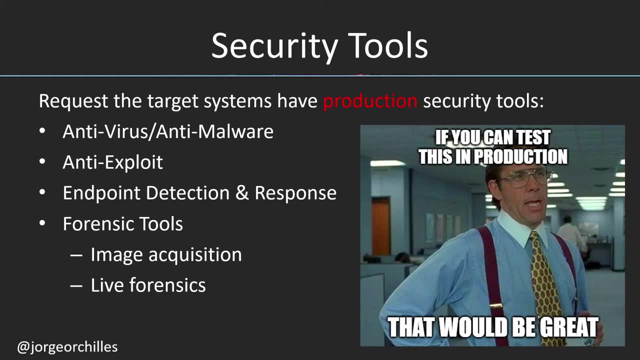 servers, windows servers. grab one or two of each so that you can do the testing. then make sure all the security tools are in there. one of the reasons we use production systems is because production systems go to production security tools. make sure you have your latest anti-virus and anti-malware running. 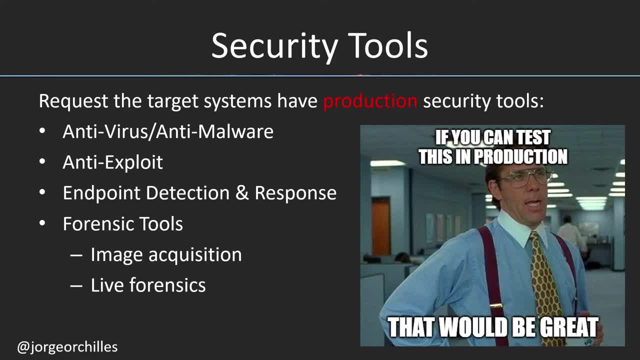 or if you have some sort of anti-exploit system. your edr solution is running, logging and uh, sending information to the right place. you also want forensics tools. now you can do live forensics or do actual image acquisition. it really depends on the timing at the speed of your enterprise tools you may want to do. 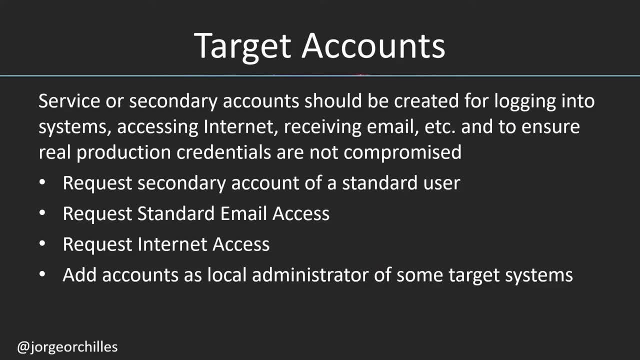 live forensics target accounts. you want to create secondary accounts or service accounts so that you're not compromising accounts of real people and having to change them. they're live. you don't want to show someone's password of a production system in front of 10 people all at once. it will. 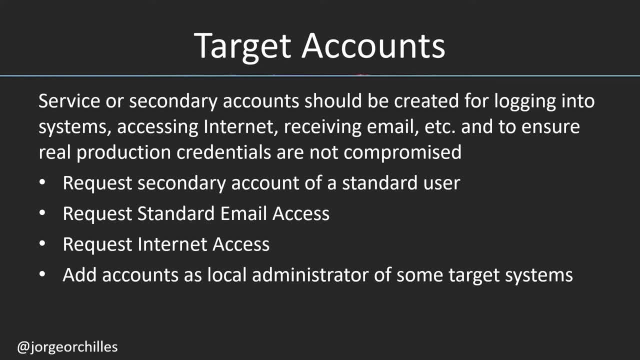 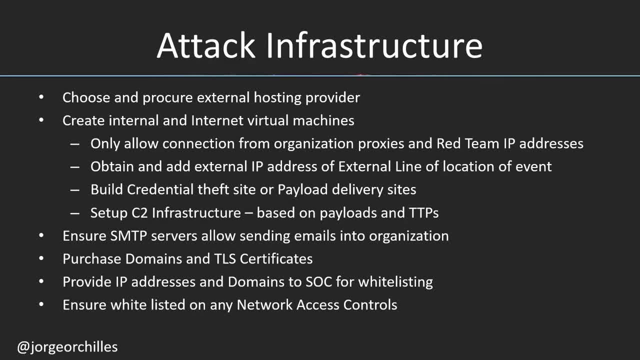 and what your goals and objectives are. attack infrastructure: if you're doing this from the outside, then you need to choose and procure an external hosting provider. you need to create virtual machines for your attack infrastructure. again, if you're doing it from the internet, you have to do certain things like add grab ip addresses. 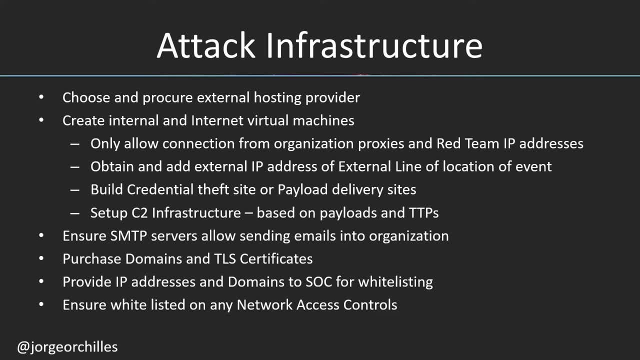 purchase domain names, purchase tls certificates- if you're going to be sending emails, you need to obtain an smtp certificate and you need to create a virtual machine for your attack infrastructure server that allows sending email into your organization. and you should provide all these ips and domains to your security operations center for whitelisting before the exercise, if you have. 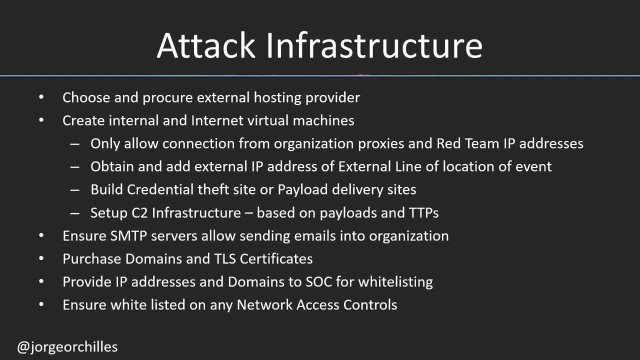 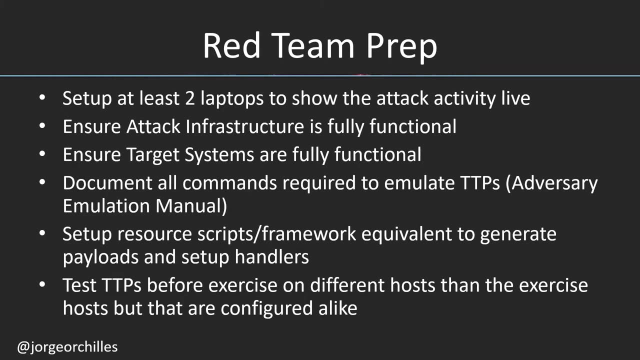 network access controls and you're doing internal virtual machines, then you need to make sure those are whitelisted as well and aren't going to be prevented. a lot of what we're going to do are things are detected, not prevented. we want to focus on detection and alerts. now the red team. 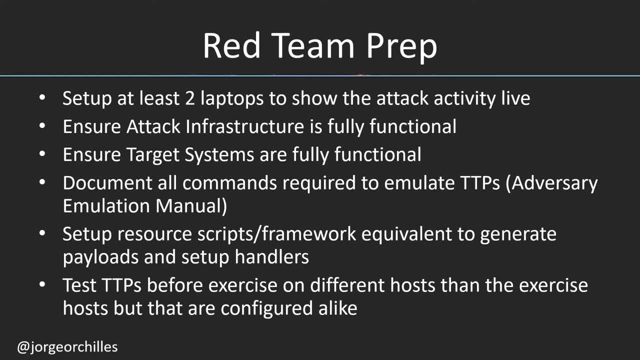 needs to prep. most of the prep will be around red team before the exercise. generally we say to set up two laptops. that where you can show the attack activity. you need to ensure that your attack infrastructure is fully functional, that the target systems are fully functional you want to document. 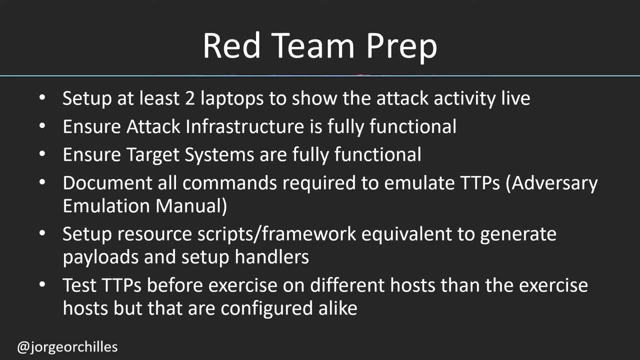 everything. what we do is pretty much create an adversary emulation manual with exact scripts and exact commands, so we just copy and paste them. we don't want hand actual typing going on. we want to do everything that's going on because that leads to fat fingering and mistakes and things might not. 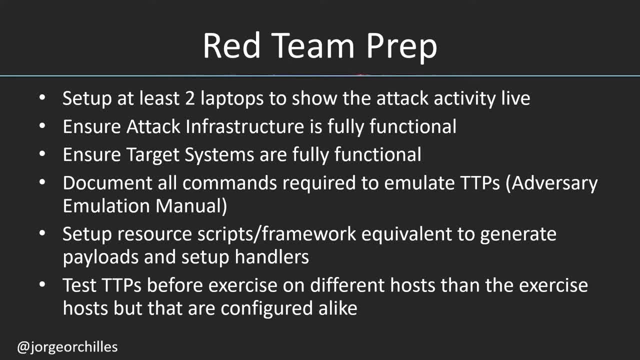 work correctly. you end up troubleshooting that instead of what you are actually trying to test, which is people, train people and process. so set up scripts or use a framework. later on, i'll talk about a product called scythe that allows you to create a lot of these ttps all in a synthetic. 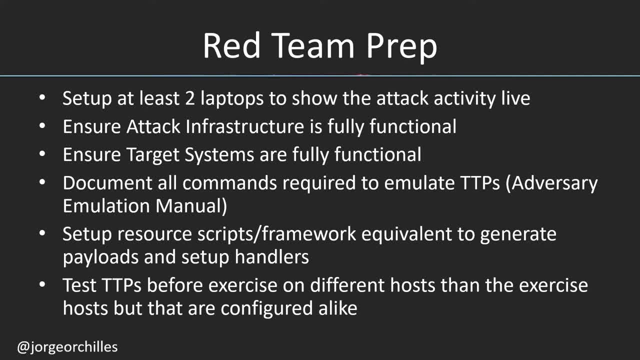 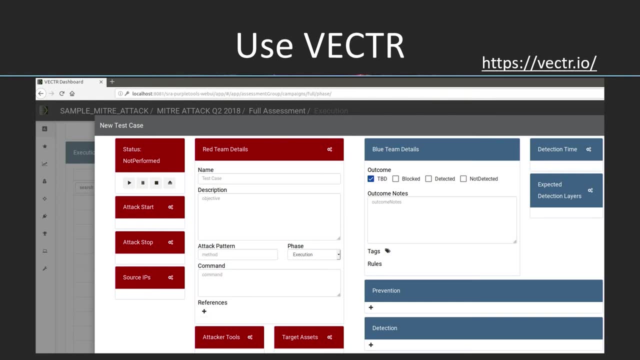 malware type of executable that you can just run and it will perform those ttps for you. Test TTPs before the exercise on different hosts so that you're not leaving artifacts on any system I like using Vector. Vector is a free tool by Security Risk Advisors. 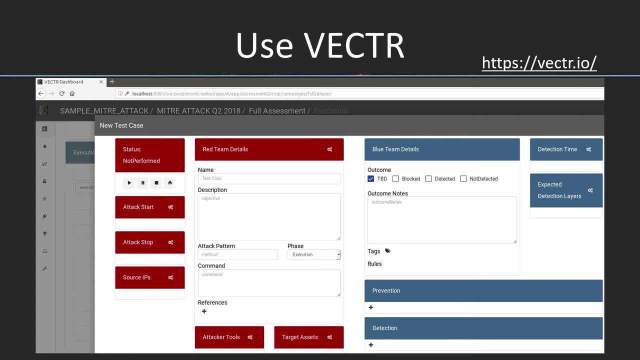 that is made for red and purple team engagements. Here you can create all your test cases before the exercise ever runs. So this is a new test case that we're creating. We fill out the red portion of this. We put the test case name. the TTP we're going to execute based on our planning. 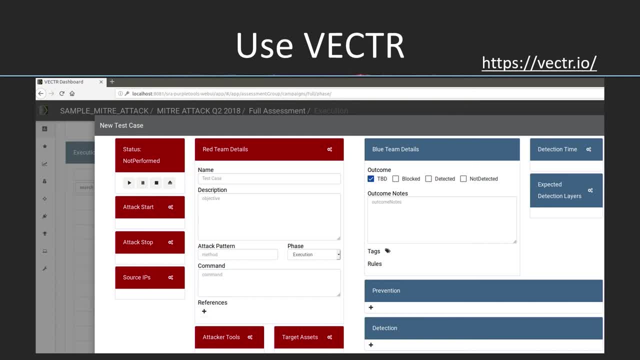 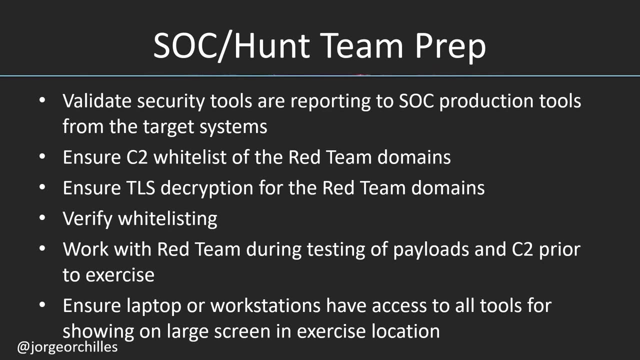 the description, the exact commands you're going to run. You can also put your source, IP and the attacker tool all before, and even the target asset all before actually getting to the in-person exercise. The SOC and HUNT team also need to prep. They need to validate their security tools are working on those production. 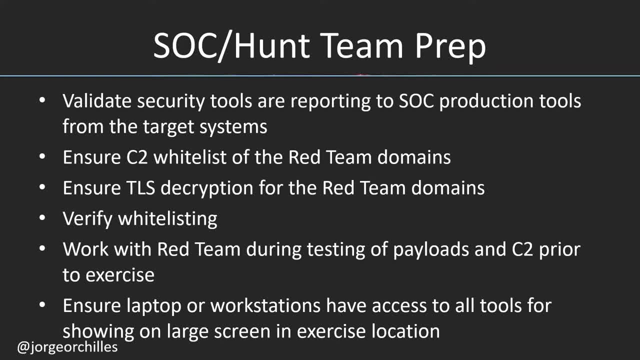 systems, that those accounts that were created are also being logged and being sent to the right places, that log aggregation is working, that their SIM is working, that they whitelisted their command and control domains the red team is going to use If they need to decrypt that as well. 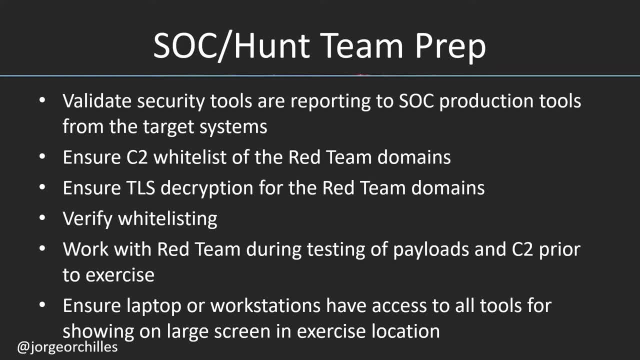 make sure that those domains are part of the TLS decryption. Just verify all those whitelists work with the red team during the test. Make sure that all of this works- not necessarily the same people that are going to be in the exercise- And then ensure that the SOC and HUNT team have laptops or workstations that they can. 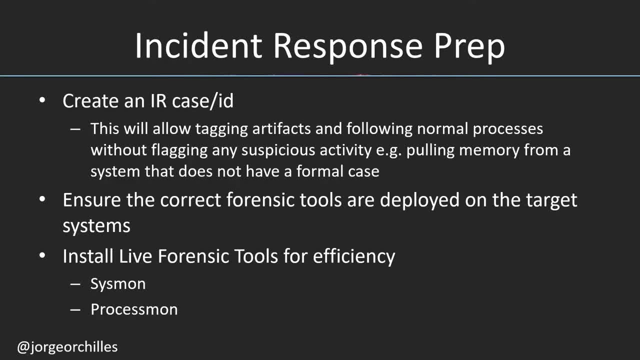 show within the conference room location: Incident response prep. Always create an incident response case or ID in whatever system you'd use for incident response. That way, you log that all of this and all the actions you're going to be taking are part of an 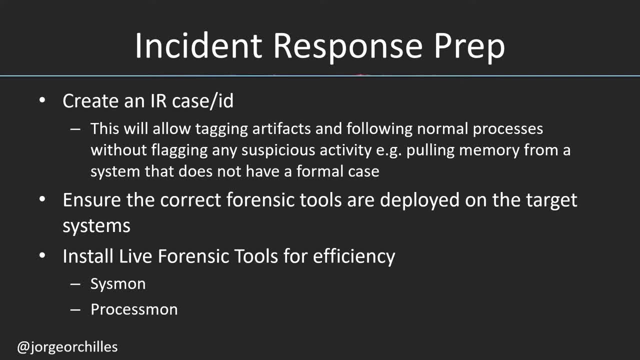 exercise Generally. you can't just pull memory from whatever system you want. All of that needs to be tracked. Then ensure the correct forensics tools are deployed on the target systems And I recommend installing some live forensic tools for live forensics, if your memory and hard drive 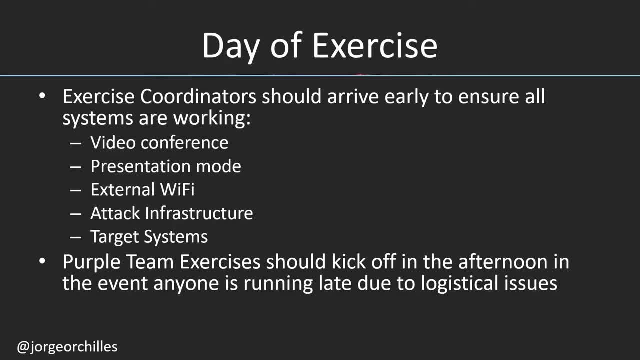 acquisition takes too long. Then the day of the exercise, We'll have our exercise coordinator show up early and make sure everything's working: The video conference equipment, the presentation mode, the Wi-Fi, the attack infrastructure is accessible from that connection, Target systems are accessible, etc. Most of the time we like. 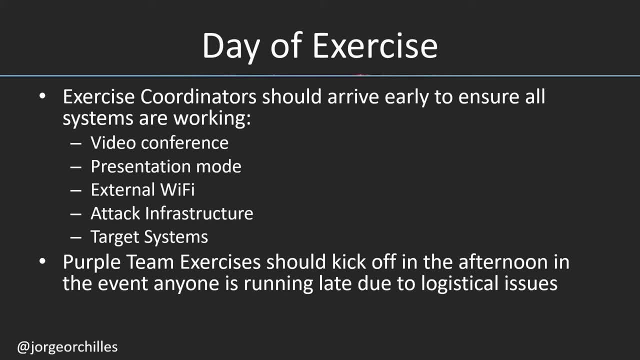 kicking. have everyone come in in the morning, fly in in the morning and then kick off in the afternoon. This will allow any logistical issues to be resolved in the morning And then we have the kickoff. Here, generally, a sponsor or more senior level person will have the opportunity to. 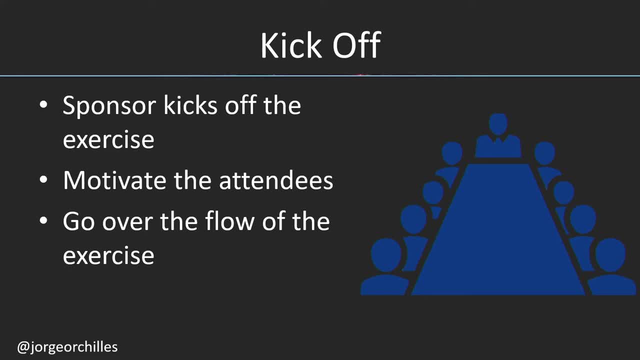 arrive and say: we are all gathered here today to do an in-person exercise. You are all the best of the best in each of your functions. We want you to cross train. We want the red team to learn what the SOC is doing, what the hunt team is doing, what the incident response team are doing. We want 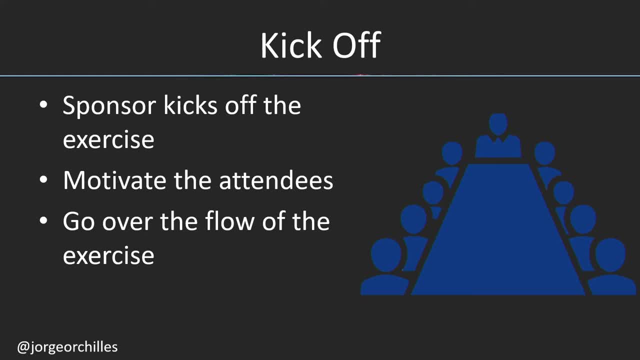 incident response, to learn what the SOC does and what red team does. We want the SOC to learn what incident response and red team do. You're all here to learn. Let's make this a nice working relationship. So you go, and then you go over the flow of the exercise which I'll present. 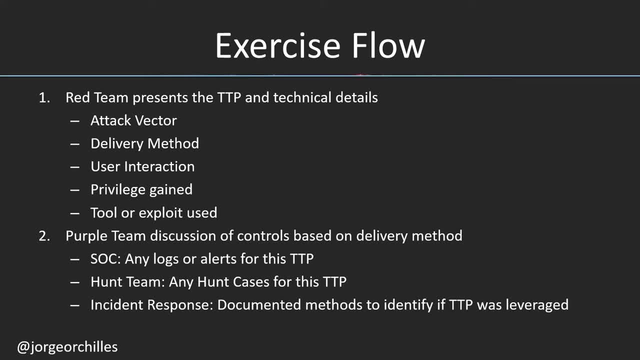 next. So what is the flow? You're all sitting together. First, the red team will present the TTPs and technical details. Maybe have someone from cyber threat intelligence give an overview of the adversary that will be emulated and the TTPs. Then, for each TTP, you look at each TTP. 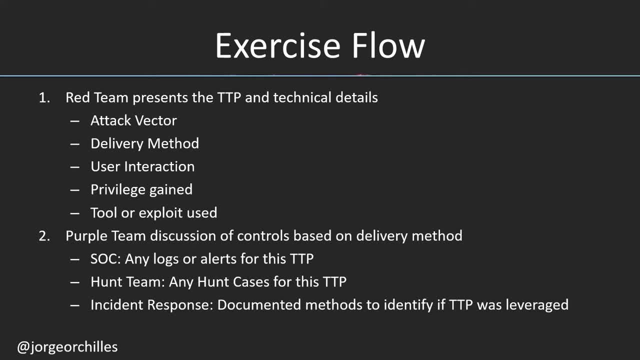 you look at the attack vector, how it's going to work, how it's going to work, how it's going to deliver, how, if the user interaction is required, if a privilege is granted, and what tool will be used, Then discuss as a purple team: what controls and what capabilities does the organization have? 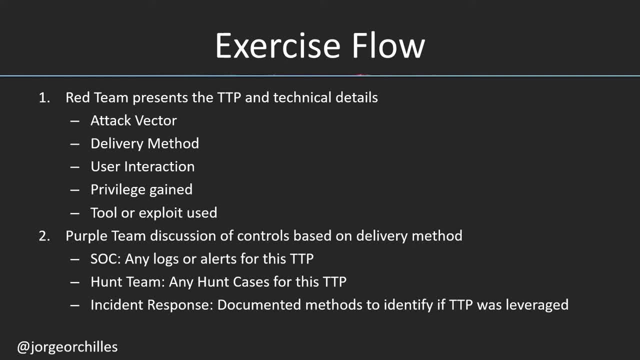 to log that information or to see that information. Does the SOC have logs for this? If it's a phishing email coming in, where are those logs? If it's an outbound HTTP request, what logs those HTTP requests? Is there network controls? Are there endpoint controls? Then the hunt team can say: 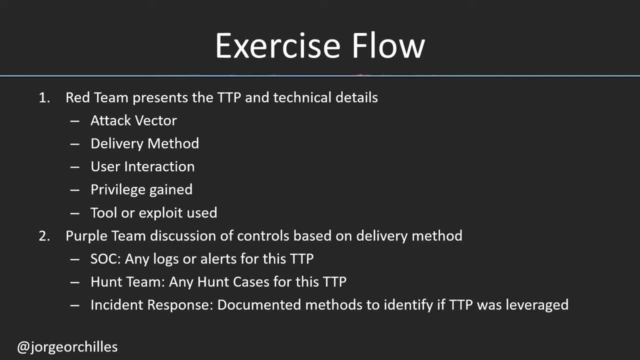 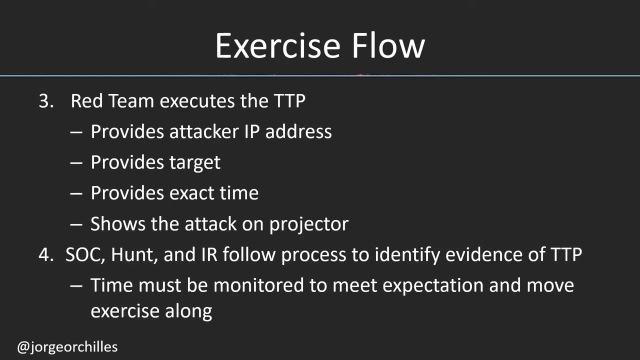 oh, we have a test case for this. This is what we hunt for, This is what we would find And incident response says: okay, if that were to happen, we would look at memory forensics and be able to determine that these actions were done. Then the red team executes that TTP. 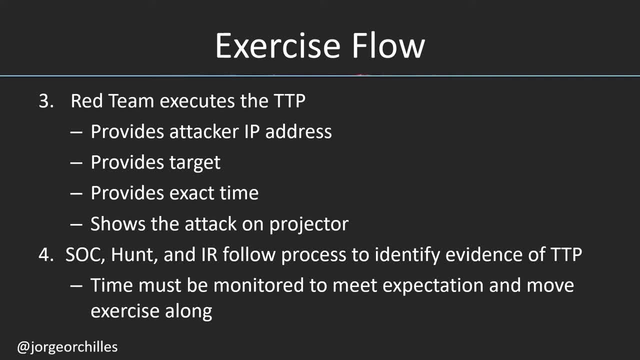 They do all of this in a non-blind format. They show the attacker IP address, They show the target, They show the execution and document the exact time it ran. And hopefully all of this works because the prep part went well and some action occurs successfully. 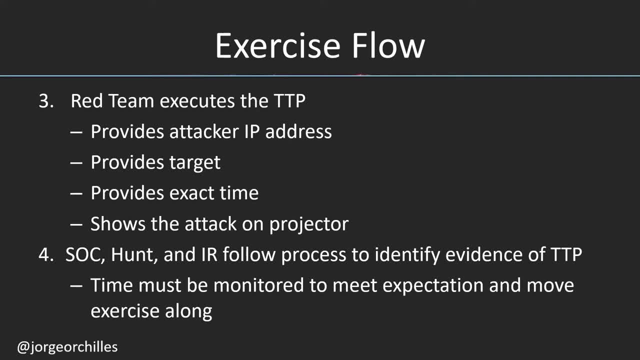 The SOC hunt and incident response will then follow their process to identify evidence of this TTP. They will monitor what alerts came out, what was logged, how quickly something was logged, How quickly an alert showed up. All of that Log, all that information, And then here you can. 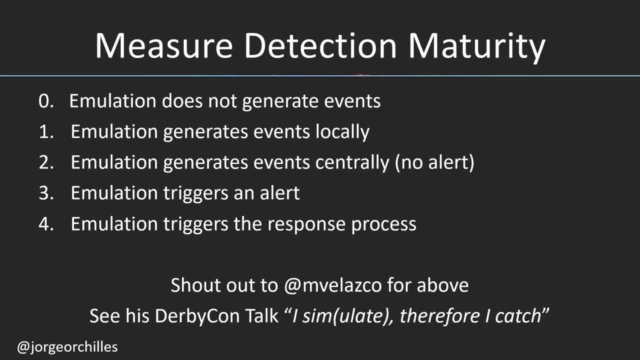 measure detection maturity. This is shout out to. Maurizio Velasco Did a talk at Derby called I simulate, therefore I catch, And he provided this measure detection maturity. model Zero means emulation does not generate any events whatsoever. One means emulation generates no events whatsoever. Two means emulation does not generate any events whatsoever. 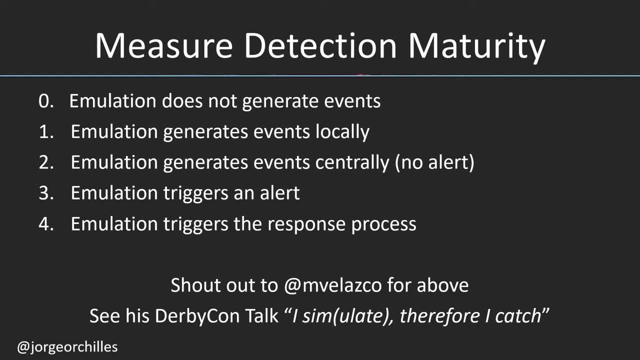 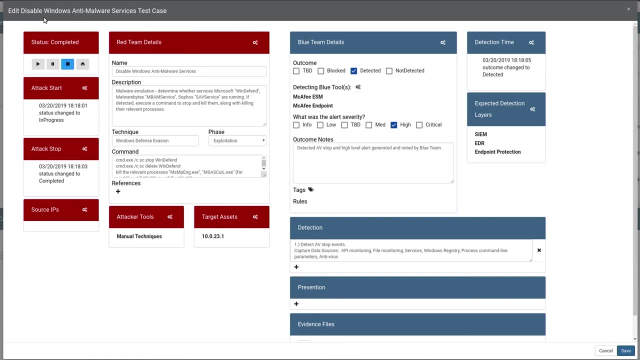 Three emulation triggered an alert And four emulation triggers the response process. It's a great way to track it. on a spreadsheet, As I mentioned, I prefer vector. So on the left side we already had this filled out. Now fill out the right side. You should already have the expected. 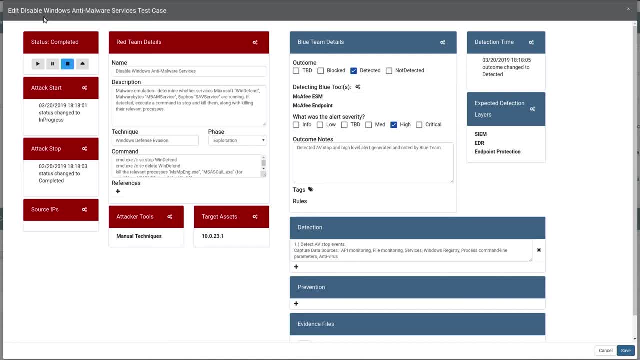 detection layers filled out, because that is what was discussed as a purple team. Then you put the outcome: Was it detected? What detected it? Was there an alert? What was the severity of that alert? And then you can put any detection and prevention and even evidence. 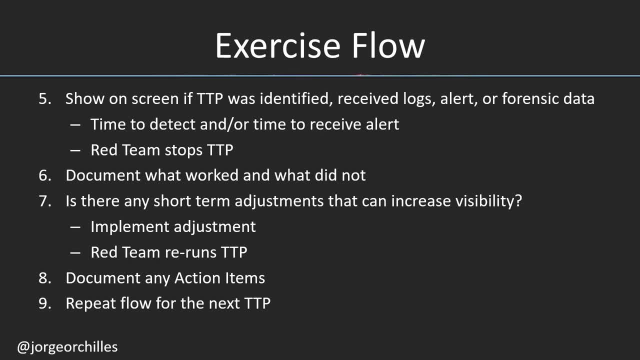 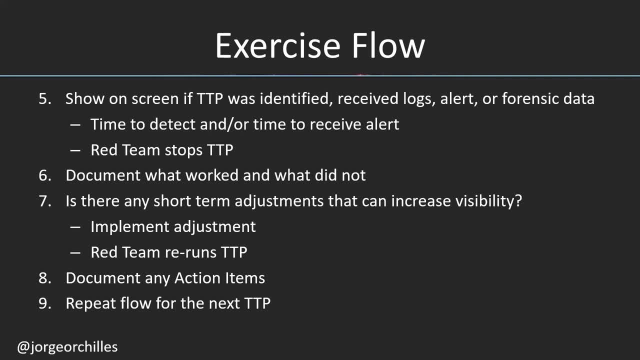 the red team is learning. Here is both teams learning. It's not one team teaching the other. Everyone is collaborating and learning. The red team will then stop the TTP Document what worked and what did not. This is the exercise coordinator's job. Is there any short-term adjustments that can? 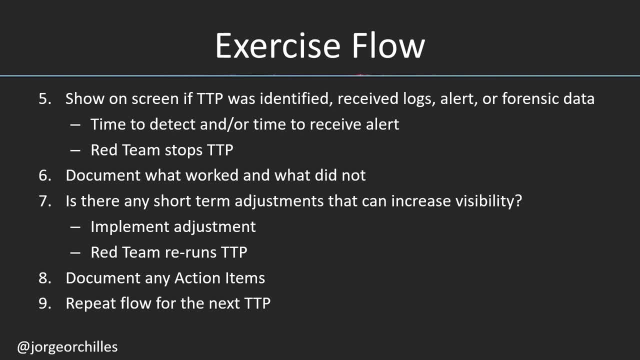 increase visibility Is something was supposed to work, but didn't. Why not? If you can troubleshoot it quickly, go for it. If not just document it. If you can troubleshoot it quickly, then have the TTP. All of this requires documenting action items. Then repeat over and over until all the TTPs. 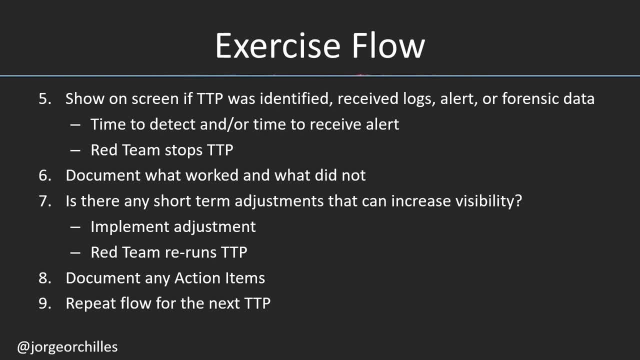 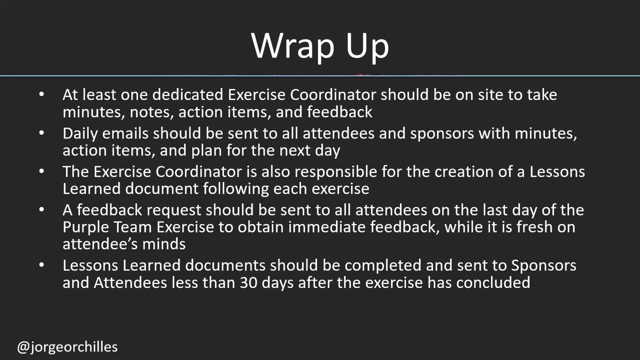 are done based on the amount of days you have available, And then you have the wrap-up. Make sure you have at least one dedicated exercise coordinator or two to be on site taking minutes, notes, action items and feedback. Daily emails should be sent to attendees and sponsors with the 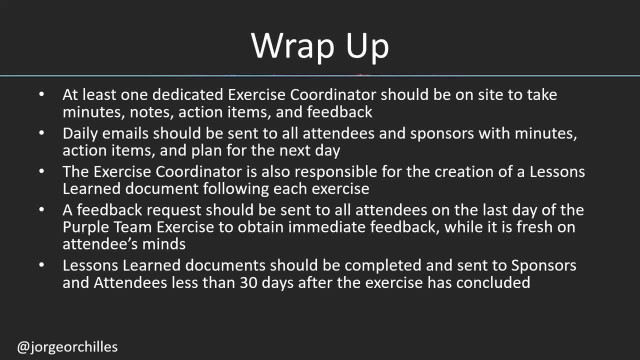 minutes, notes, action items and feedback. If you have any questions, feel free to email me at. The exercise coordinator will also be responsible for the creation of a lessons learned document. They should request feedback from each attendee at the end of the purple team exercise to see. 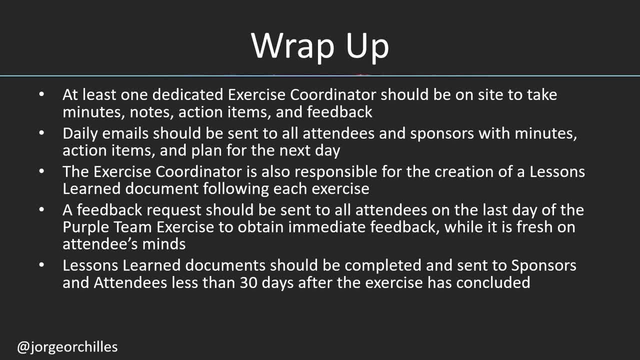 how it went. Do this right after, as everything will be fresh on their minds. Most of these people just took a week off to do this. If you wait a week, they will be head deep into something else and not spend the time to do it. And then the lessons learned. documentation should be completed. 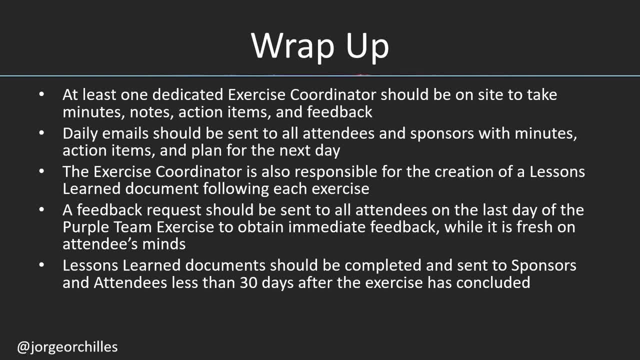 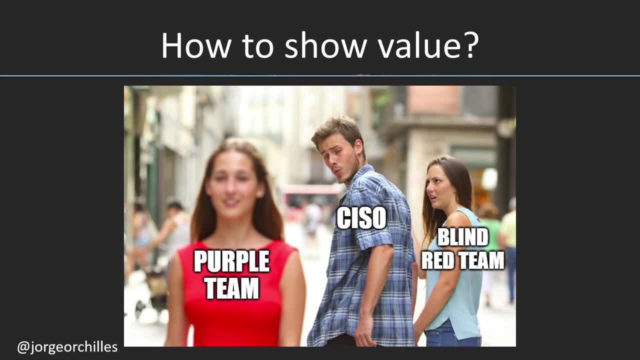 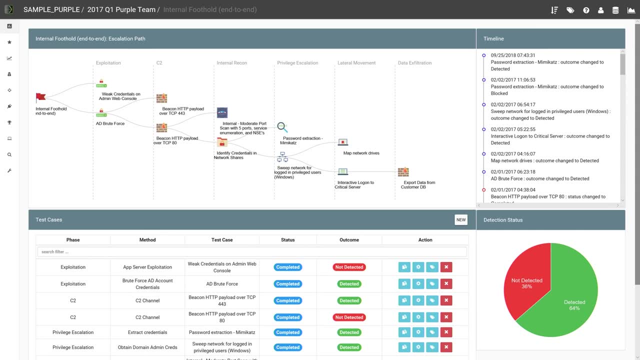 and sent to sponsors and attendees less than 30 days after the exercise has concluded, And then track all of this. So how do we show value? As I mentioned, we can use vector. If we use vector to create test cases for each TTP, then we can look at our report. If we use vector to create test cases, 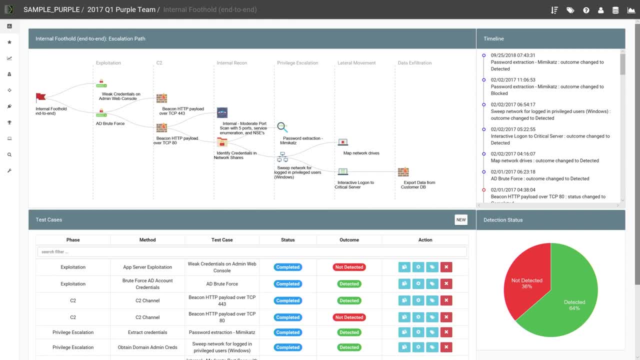 at the reporting functionality in vector and see screens like these. On the top left you have each TTP mapped to the cyber kill chain. This helps quite a bit because that's what senior managers or senior management knows. That's what they know works the cyber kill chain. On the right you have 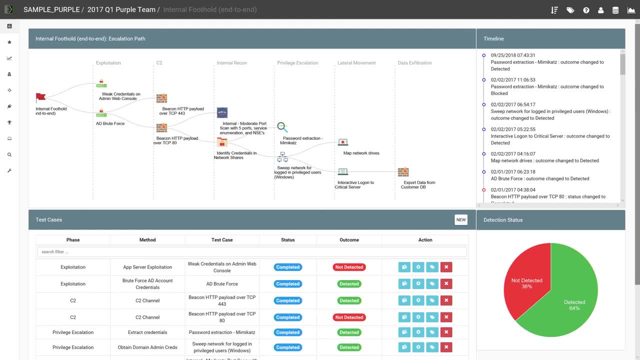 a timeline of what occurred, at what time, both from the attack and defense perspective. You can see both blue team and red team. And then you have a timeline of what occurred, at what time, both from the attack and defense perspective. You can see both blue team and. 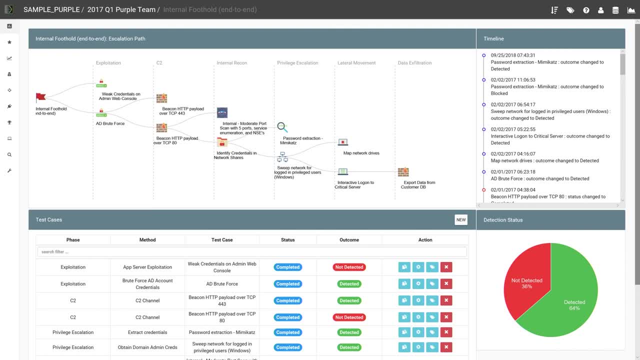 red team. there on the bottom You have your test cases, which ones were completed, what was the outcome, And you can click on each one to get more details. And on the right you have a nice little pie chart that anyone can understand And it simply says that 36% was not detected, while 64%. 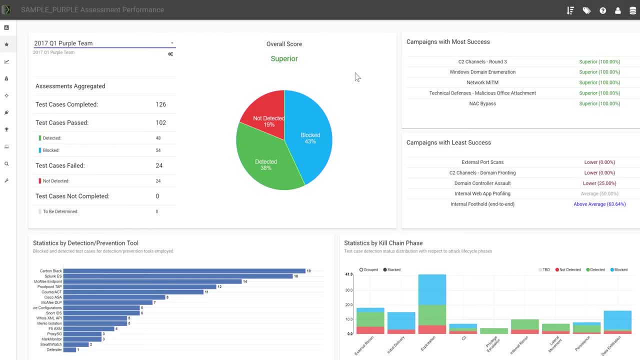 was. That's actually very good for an environment. Here are other methods and other reports that you can take a look at. On the left you have a timeline of what occurred at what time, both from the attack and defense perspective. You can see. 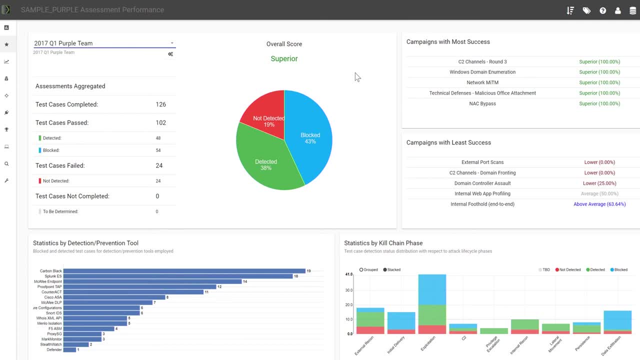 the left side, top left, you have all the test cases you've completed, with a nice little pie chart of what was detected, not detected and blocked. On the right you have the campaigns you've ran. You have which campaigns ran with the most success and the least success. On the bottom left you have 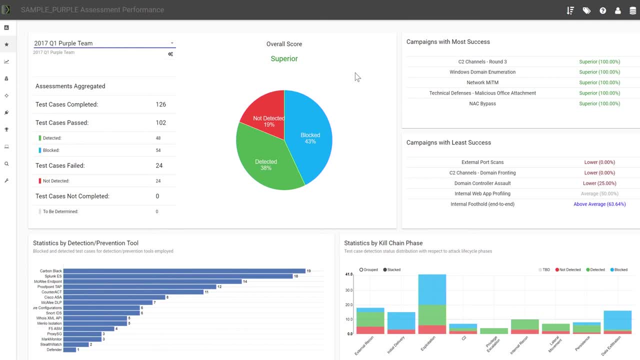 statistics by the detection and prevention tool. This is great for engineers to see which of their products provides the most value against an adversary actually attacking you, And on the bottom right you have a timeline of what occurred at what time, both from the attack and defense perspective. You can see. 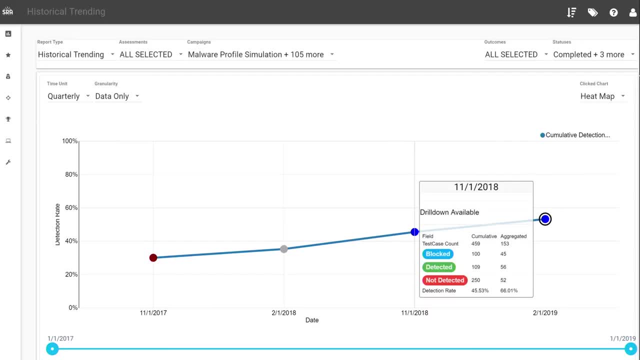 the left left side, top left, on the top right. here you have statistics by the kill chain phase. You also have historical trending, which is really nice. You can show how you have progressed and improved. In this case, we're looking at the detection rate and we see that the detection rate is growing. 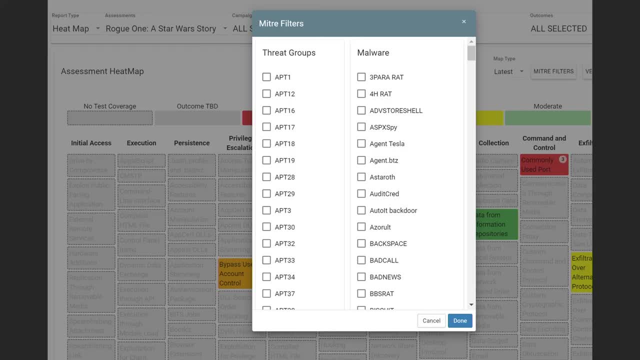 assessment over assessment. We also have the ability to filter by threat group, And this is awesome. if something like January 2nd occurs, where the Iranian threat actors are now the question that all senior management wants to know: What can Iranian threat actors do to us? You can actually filter here by the threat group. 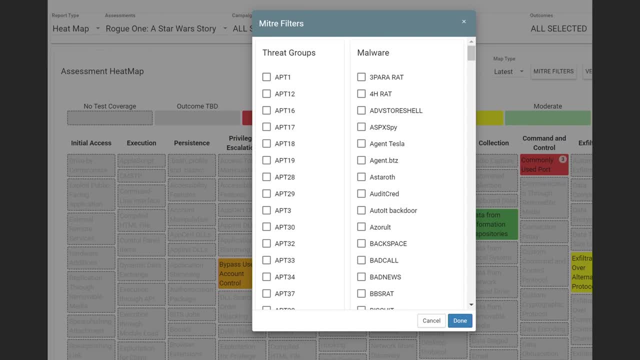 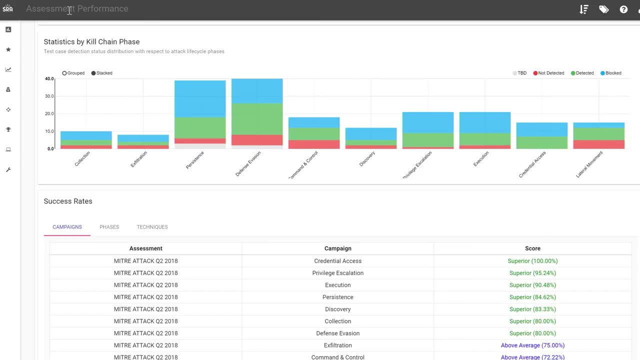 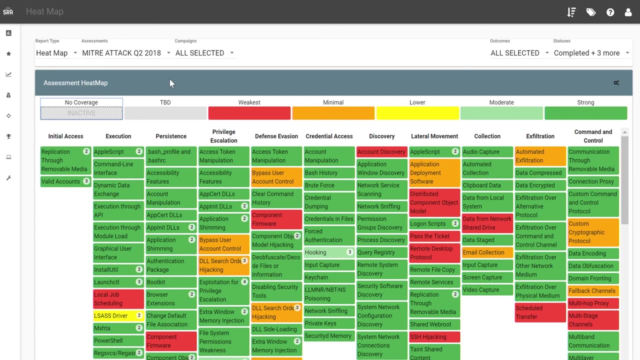 and have a heat map of the various different TTPs you've already tested. along with the coverage, You have statistics by kill chain, which I showed earlier. This is just a bigger screen and a heat map of what it looks like Now. there's a lot of green here Generally. 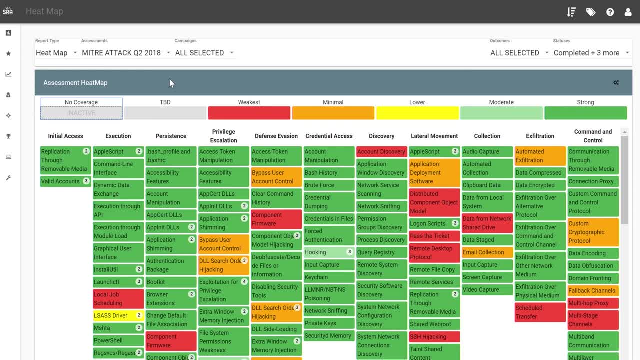 you will not have a lot of green. You'll actually have a lot of red, which means you have no detection whatsoever. You may have some alerting and some actual prevention. Now the question I always get is: I don't have a red team. What do we do? I want to do this type. 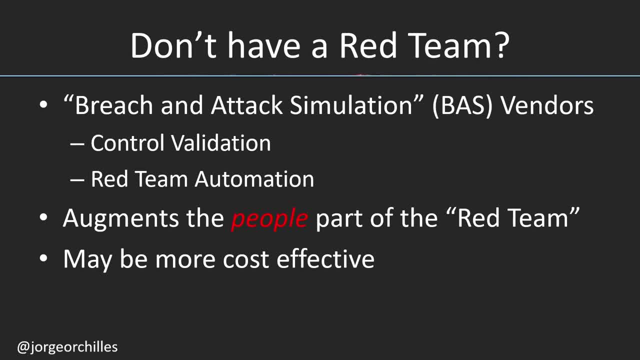 of testing. Well, there are vendors out there called breach and attack simulations. A lot of these do more control validation, where they will replay a same packets over the network and see if the detection is continually working. Others actually automate these adversary emulations and the TTPs being performed. This really only augments the people. part of the red team. 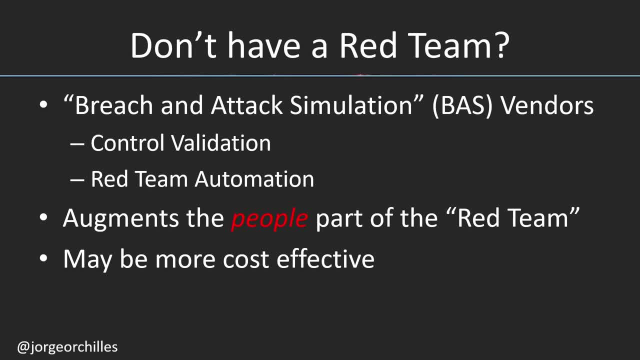 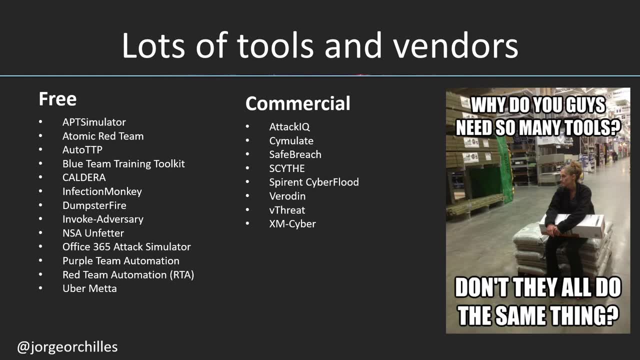 And no, this does not replace an actual red team, an actual person. So there's a lot of tools and vendors out there. There's many free tools available from on here, as you can see on the left, and many commercial tools. I can go on for days, as I spent a lot of time looking at all. 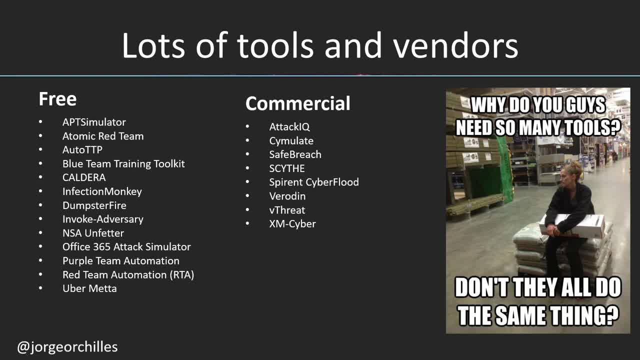 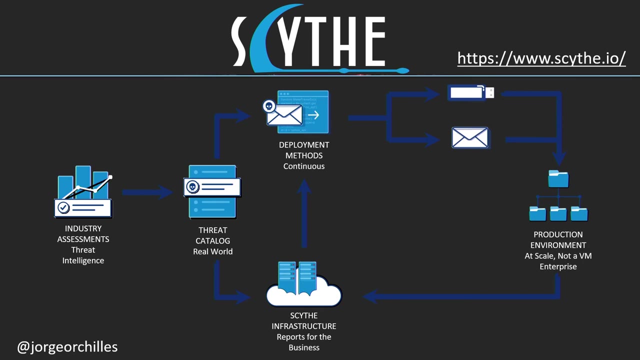 of these. We'll leave that for another presentation, But I just want to show, because this is how most of these solutions work. A lot of them do replays. They don't actually run the TTP. There is a vendor, though, called Scythe, that does actually emulate these TTPs They obtain. 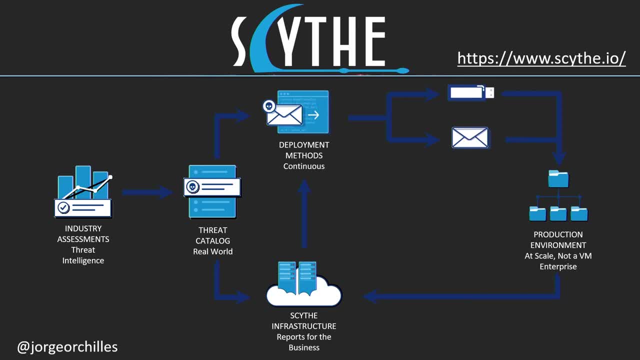 the threat intelligence. As you can see here, they have a threat catalog And you can actually select all the TTPs you want to run, create a payload and deploy that payload in the production environment. So the payload is generally an executable or a DLL. You execute that in one. 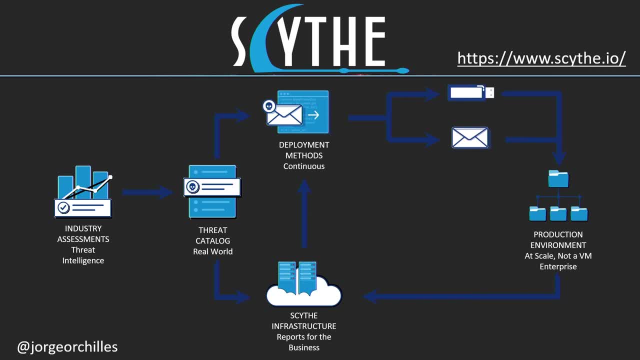 place, As if someone fell for a phishing email, And it will execute the TTPs you have selected. It has the capability of working with atomic red team as well, So it has a lot of TTPs that you can emulate And then it reports back And you can correlate all this with your different solutions. 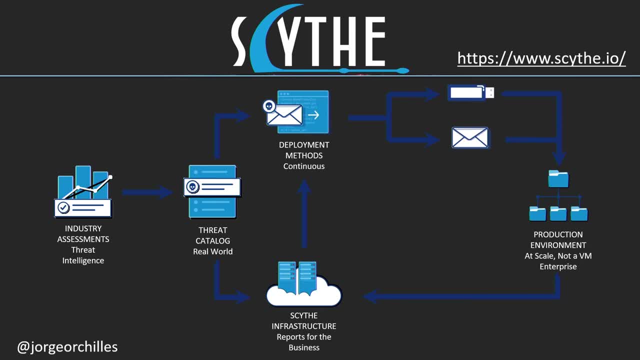 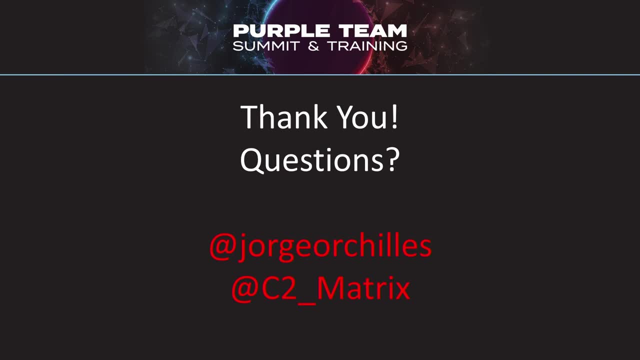 This, of course, is just one of the solutions available. Check them out And, of course, interact with me on social media If you have any questions about any of this. also the project lead for the C2 Matrix. So I am. 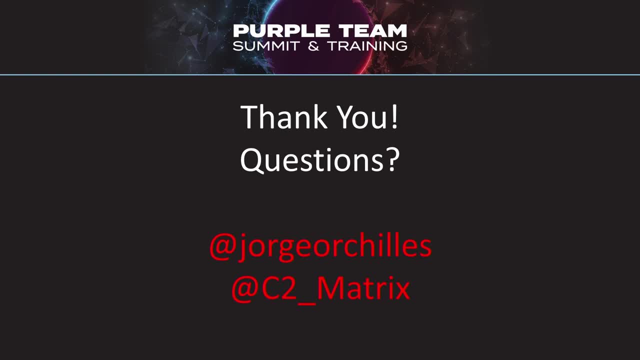 available to talk about all this stuff. I love it And I appreciate your time for coming here and listening to this talk.